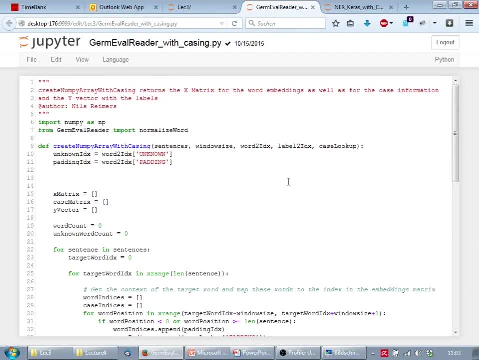 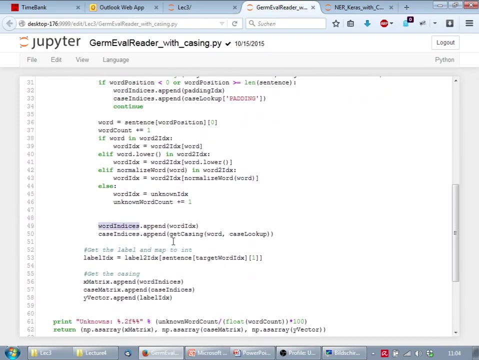 for the beginning is like: yeah, first like an array with our word indices and then we need a second matrix with, like, the case information. So we adapted our preprocessing So here it creates a NumPy array with case information And here we have, like, we have like a list, an array, a matrix for the word indices and 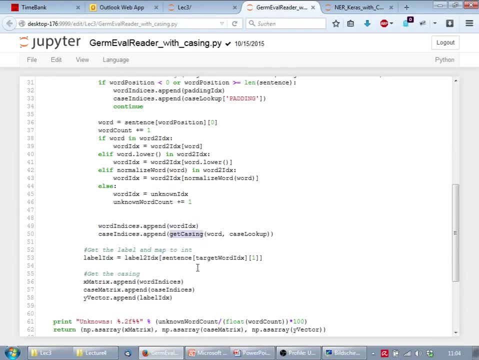 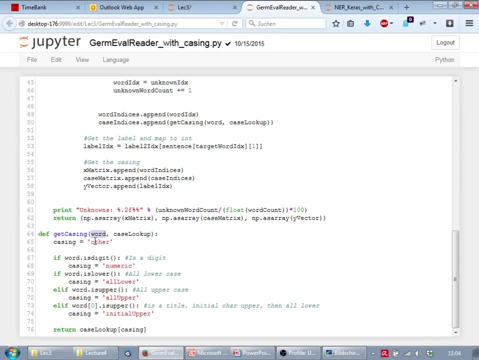 the same we get for the case indices, where we have, like a function, getCasing, which gives us the casing for a word. So here we have the word, and then we can say, okay, it's ether, so now define casing. 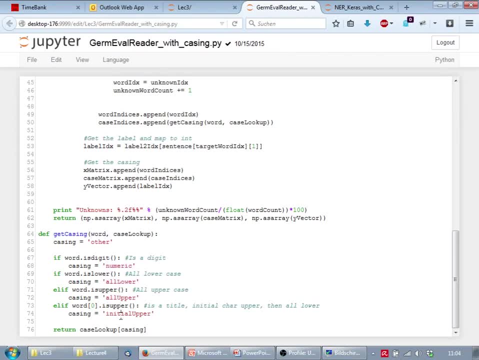 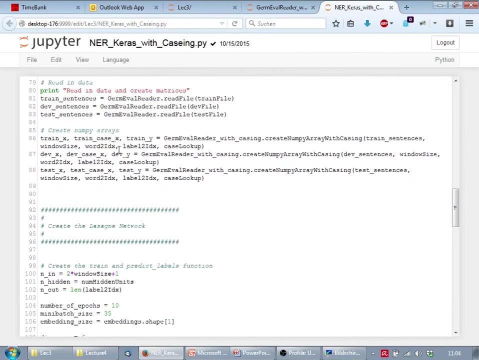 Or it's like: is it a digit? Is it lower or lower or upper Initial upper? And we just return like the case information. So which of the cases is it? And to implement this in Keras. so what you need to change is: here we get now a train matrix, a matrix with the 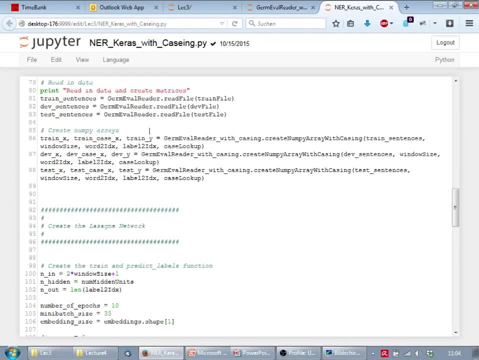 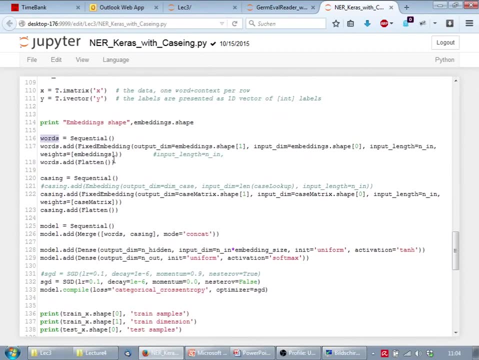 word indices and a matrix with the case information and the label for the training. And what we model is. We have a model for the words which is like an embedding matrix with the word embeddings, And we do the same with like for the casing. So we define a model for the casing where 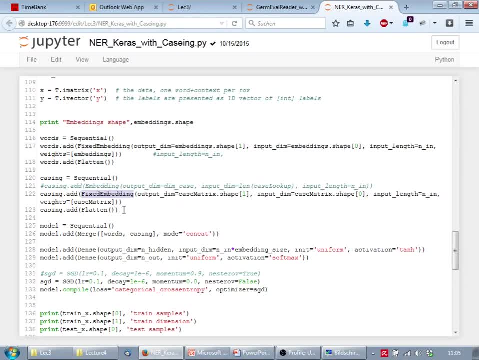 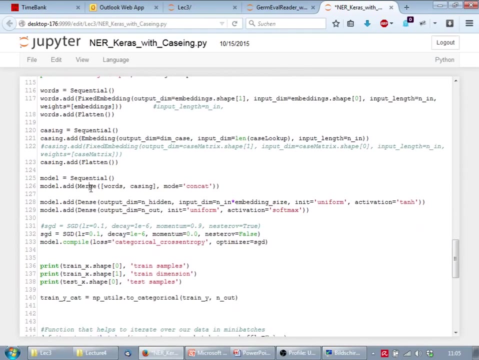 we have like a single layer. Either we can say we have a fixed layer if we have like one fixed embedding for the layer, or we can also update it during training, where we then just select the embedding matrix And our final model uses then the merge operation. 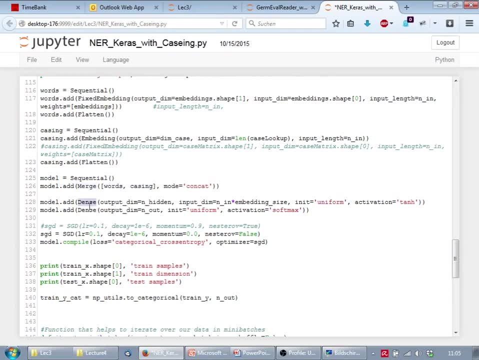 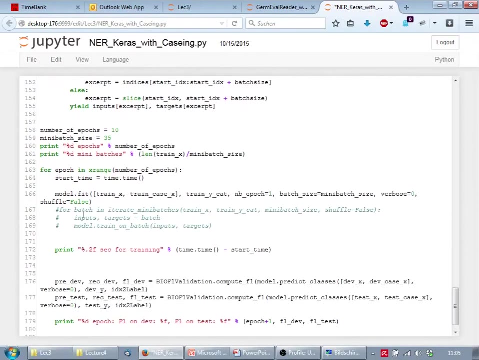 And which merges the words and the casing, Adds like a dense layer, a hidden layer, a softmax layer, And then we can run our program on the SGD. So we can compile it, we can train it. And for training we say modelfit and we input train x and train case x as the two. 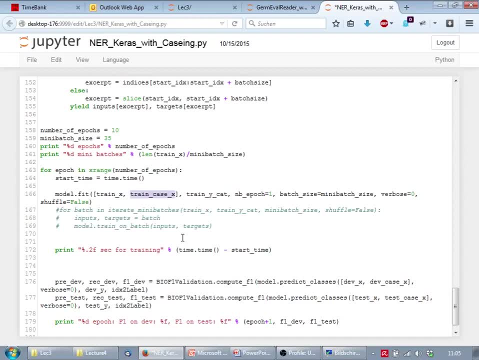 inputs of our model. So train x was the word indices for the first model and was the case indices for the second model, And as an output we get the information. So if you have like different features, for example, you want to add, like also part of. 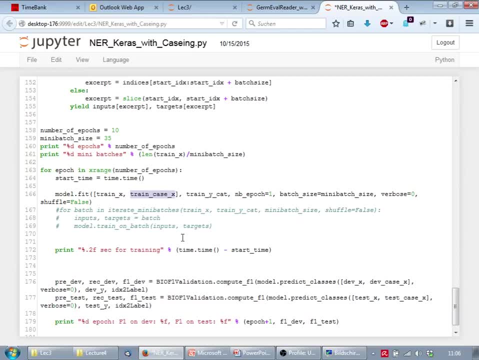 speech into your model. you would just define like a third model, And then for every model you can define: what do you want to do. So typically you just do an embedding, But you can also do like more complex stuff on every part And at some point you out merge the. 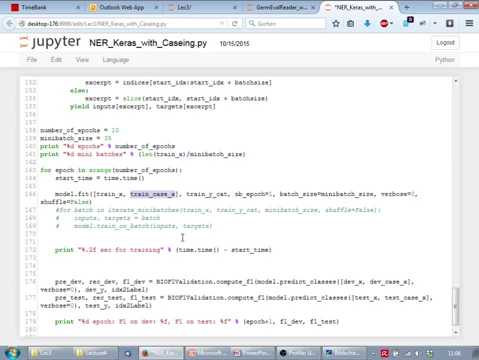 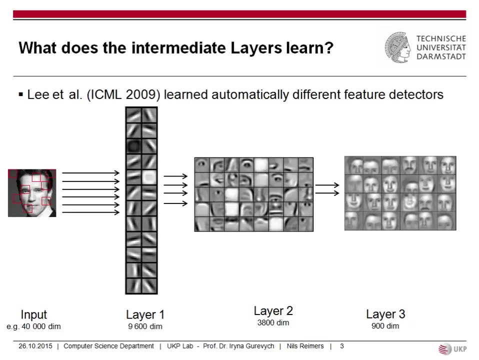 output for all the models. Okay, last week we had the question: what does the intermediate layers learn And can we derive some meaningful interpretation out of it? And computer vision, you can really nice visualize what the intermediate layers are learning. So Lee published in 2009, a 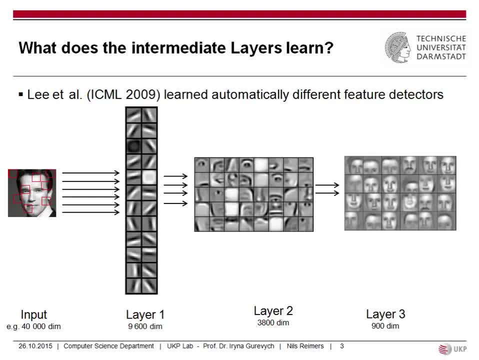 paper where he trained a deep neural network for object image, object recognition. So here he trained it on face images And in computer vision. you do not take the complete image into account, Like you just take smaller subparts of the image. So, for example, only nine times nine pixels of it. 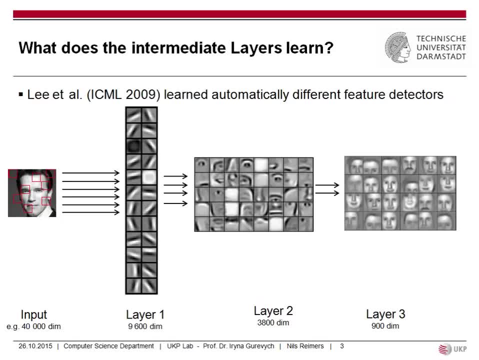 into account And then you do a convolution layer. That's some details we will cover next week and what you can visualize what the different neurons learn. So here we have, like I think these are 24 neurons for the first layer And everyone is trained on like nine times. 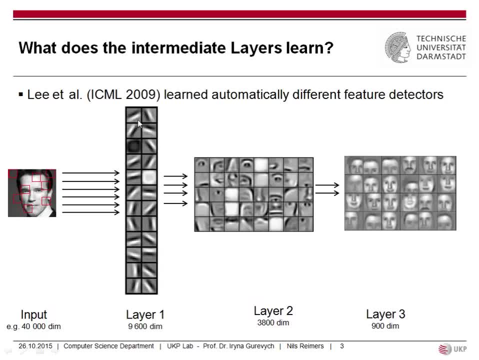 nine pixel image And then you can visualize. what does this neuron, this single neuron, learn? and this single neuron responds to an image patch where you have an edge. so you have here some dark color and then it goes over to some bright color. this neuron responds to like a black patch, this one to white patch, and then you 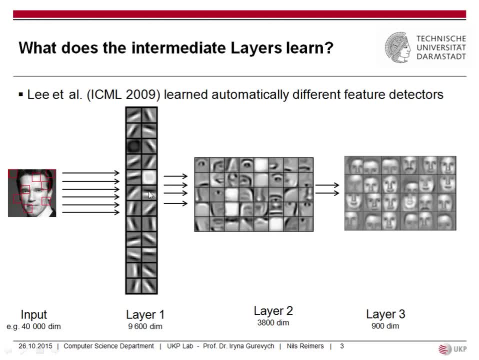 have like here in horizontal edge, from white to black. here you have like from black to white, and then all the neurons in your vectors are like white from black. Then these neurons are mapped to like to the next hidden layer, the second hidden layer, and then you can also visualize what is the. 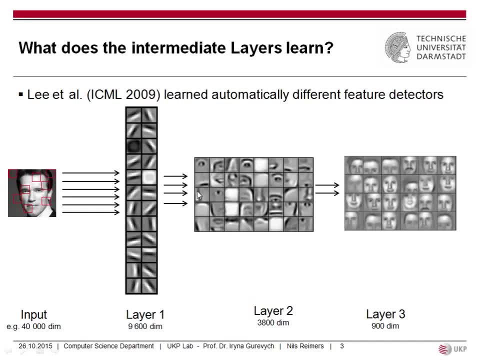 second hidden layer, learning. So here you see, okay, this one is learning- or to detect an eye- here you can see its nose, mouth, nose again, and then these are like mapped to the third hidden layer. and the third hidden layer learns to detect different faces. so here we see some female faces here, like 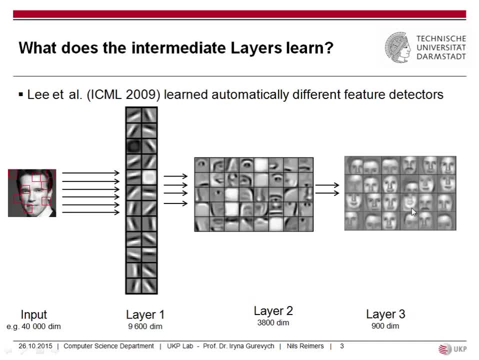 male face with mustache, And this is like automatically learned by the neurons. So no one was sitting there programming. I want to write like an edge detector, or I wanted to write an eye detector, nose detector, but the network figured it out by itself. 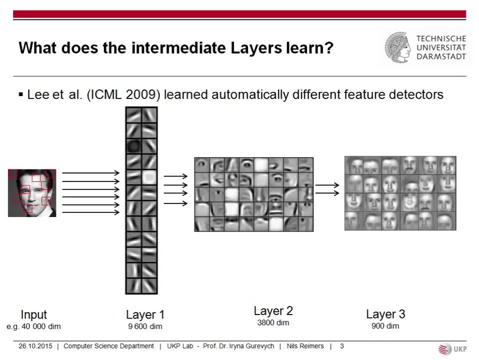 and got to this representation that when you want to detect faces, it's a really good first step to detect edges, then to detect like parts- eye, nose, mouth- and then in the final layer, to detect the whole face. Doing this for words is a bit more difficult. 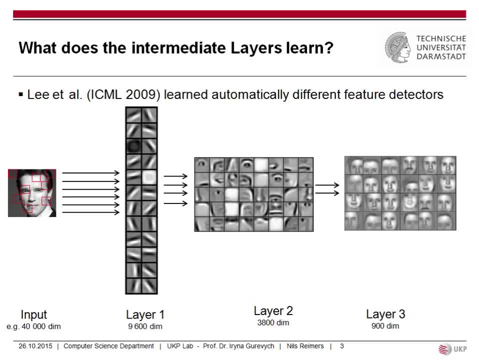 especially when you have also like the dense vector representation in between. But for images it's really nice and really straightforward and you can find a lot of these representations. Maybe when someone is interested you can also try to do the same representation for words. 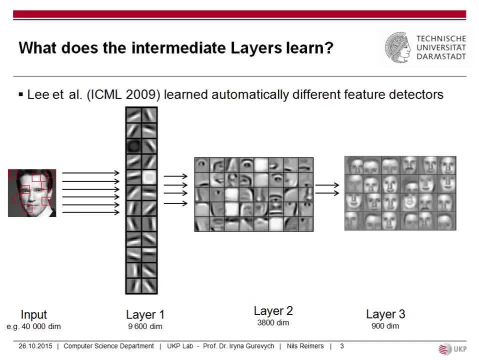 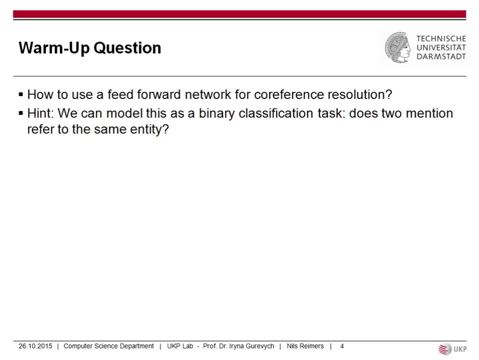 which would be like a nice, interesting research question. How can you visualize what the intermediate layers are learning in a deep neural network when you use it on, And how do you interpret it then from the perspective of a sentence or a document level? Okay, one more question. 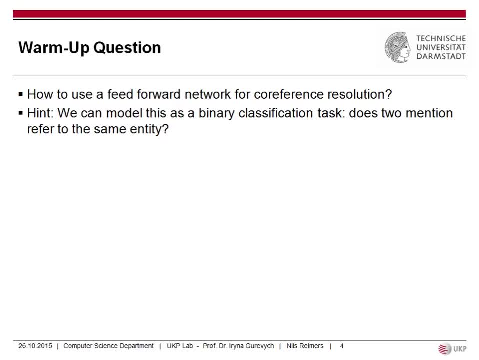 There are sadly no screws in my laptop, so that's not the stable installation. One more question: You have the task of coreference resolution. So you have a text and you have different entities and pronouns in the text and you want to establish 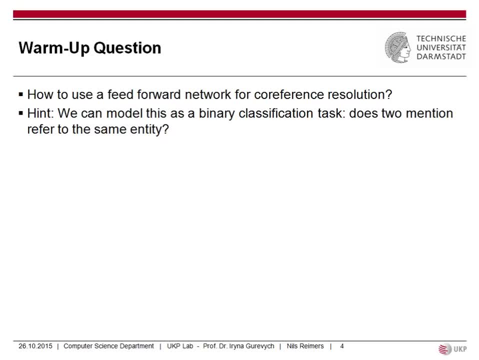 all entities and pronouns which reference to the same entity. so you have a text. obama visits illinois, he gives a talk and the president was invited- 2012 the last time- to illinois, for example- and you want to identify if these are the different chains and you can model this as a binary. 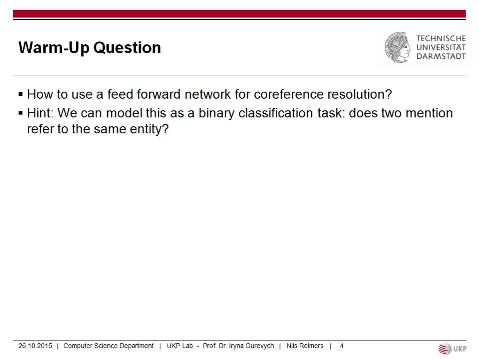 classification task. so you look at two pairs, so two mentions or two pronouns, and you try to establish: do they refer to the same entity, yes or no? and is someone willing to say okay? how could you create a neural network for this? how could it look like? how would you model it? 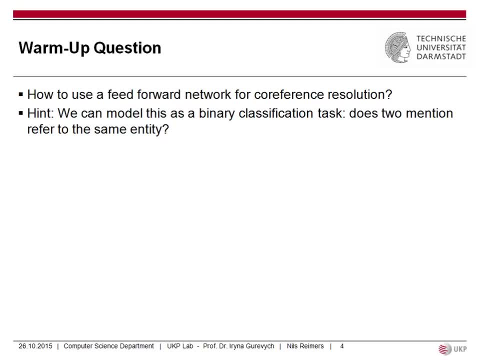 so someone likes to take a pen and draw on the flip chart for it. do you know the entities in advance? i mean, do you know where the occurrences are? so you know the entities in advance and then you try to you give your input or combinations of two. 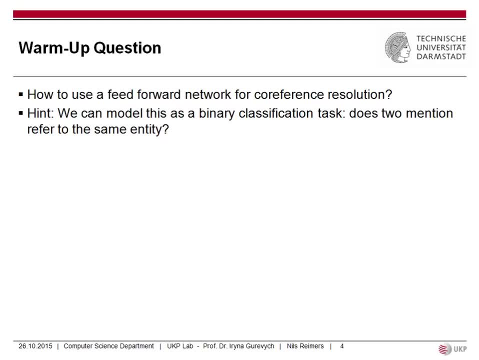 into the model and then you just try: is it the same entity, or is it referring to the same entity or not? So it's Obama and the president referring to the same person in this text And you can use deep forward networks, really similar to the network we presented last time. 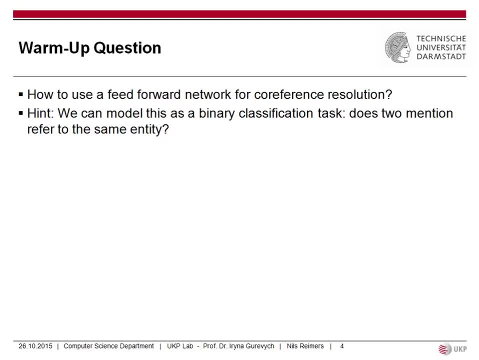 for named entity recognition, part of speech and so on. So someone you want to draw, Not yet, Not yet. Okay, What if you take the context of one entity and get embeddings on that and compare it with the others, like context of the other entity with some context? 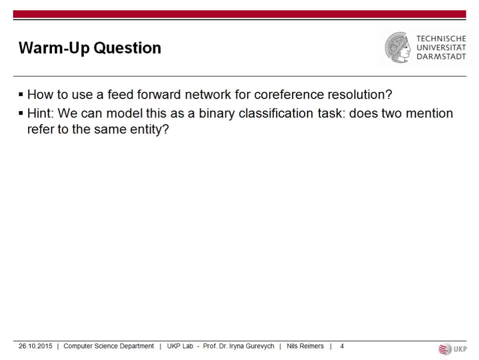 put it into one vector and feed it into it. would be like an input layer. then do some 10 embeddings. that probably gives two layers sigmoid- sorry, softmax- at the end and get this order out. Okay, yeah, That's a really good start. 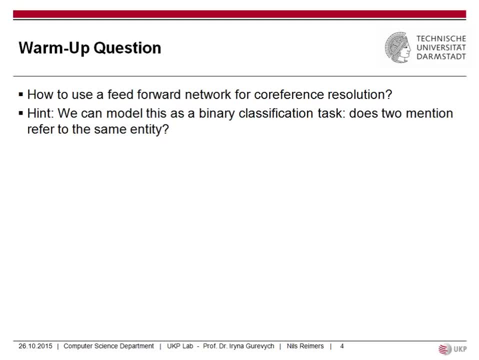 So how could we improve this model? So basically you say Like continuous back and forth. basically, Oh yeah, Context one, context two, Something like this, Something layers, Yeah, yeah, sure, Okay, How could we improve this model? or what's like. 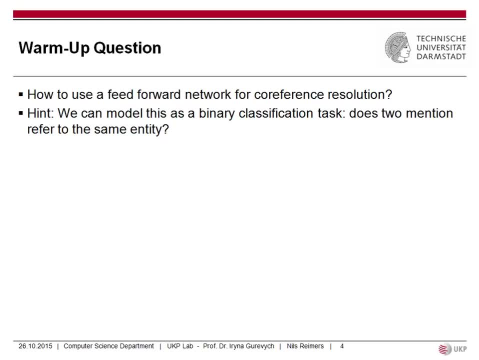 what could be an issue with this model? How do we detect the attributes of the? I don't know if they are the same or not. Maybe we try to take some vectors here. distance of the vectors, I don't know, but some in the end. 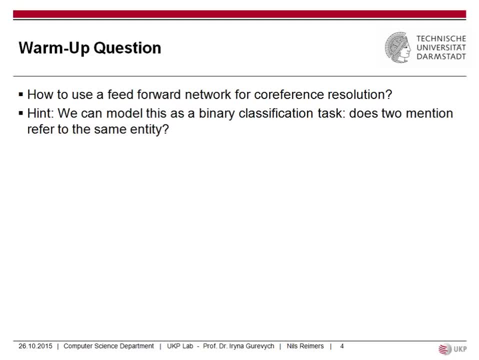 Some distance. okay, So distance is good word, but not completely correct yet. Any ideas, Further ideas, Random ideas you have in your mind What is it, pronouns and what entities are in the input? So yeah, you have entities and pronouns as an input. 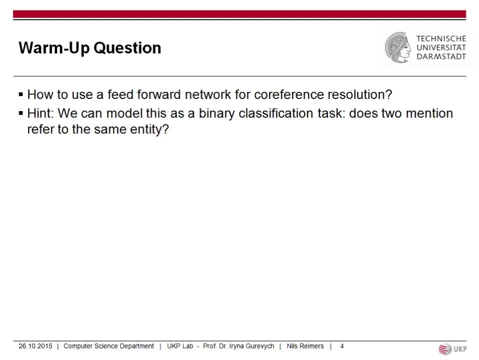 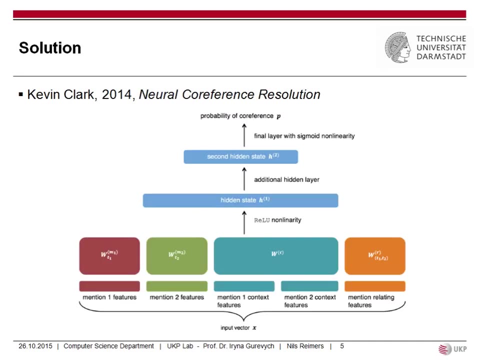 So, when I understood correctly, you put in the entity and pronouns and the context of it, do like the word embeddings and then input it. Okay, so there are some more tricks. So there's a paper from the Kevin Clark, So it's not a published paper. 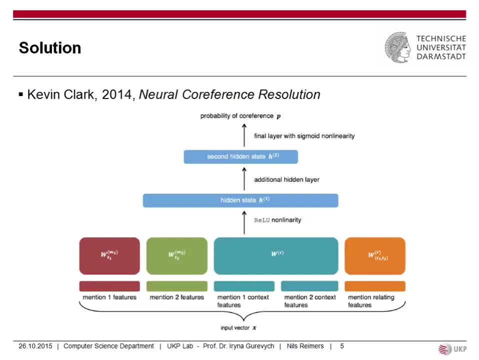 but it was class project in CS224D, the Richard Zochach class, And it's so. what you do is like you have your mention one and mention two and you take the word embedding for mention one, So you take the word embedding for Obama. 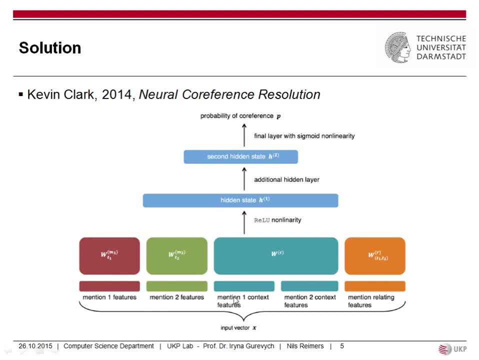 and you take the word embedding for president, Then you have some context information, So maybe the words to the left, the words to the right, you also put it into, And then you have some mention relating features. So, for example, what is the distance between the words? 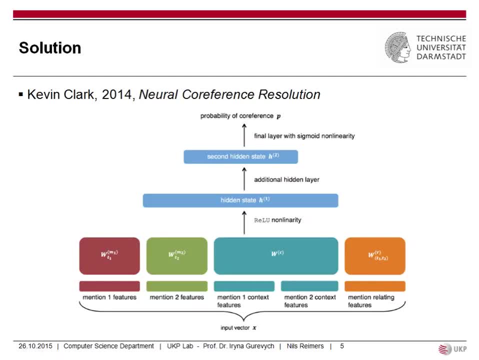 So how? what are like how many tokens or how many sentences are apart. So when you- I don't know- when you have Obama in the beginning of the sentence and he is like 10 pages later, it's not so likely that Obama and he are relating. 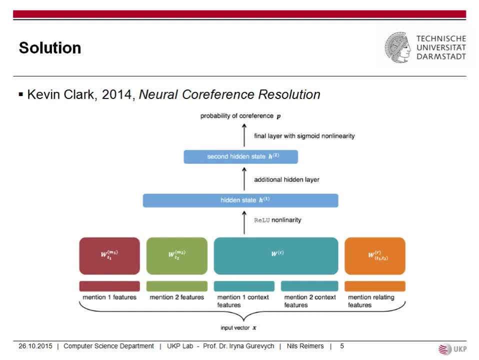 to the same person, but when he is like recurring in the next sentence, it's more likely. So you have to So mention itself. you have the context and how. what's the distance between them? You do embedding, lookup, input it to a hidden state. 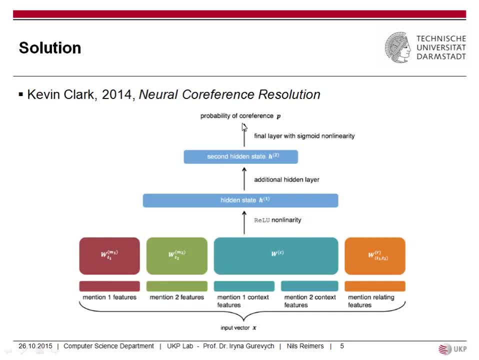 maybe second hidden state, and then you get to do a probability, So zero, one probability or probability between zero and one that these two mentions could refer to the same entity, And then you can just use back propagation, train this model. So this is like on two contexts. 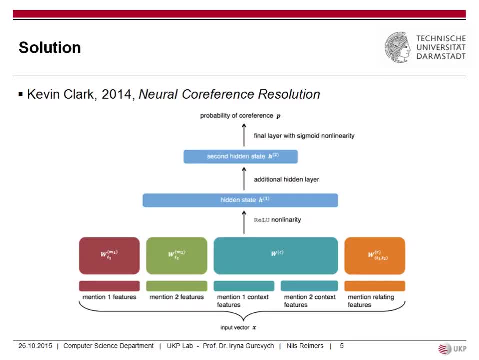 What you can also, then well, this is like the first step. What you can do is like: then, for every pair, you can establish a probability that this pair co-refers to the same person, And what we want to do is, like, typically, a chain and co-reference resolution. 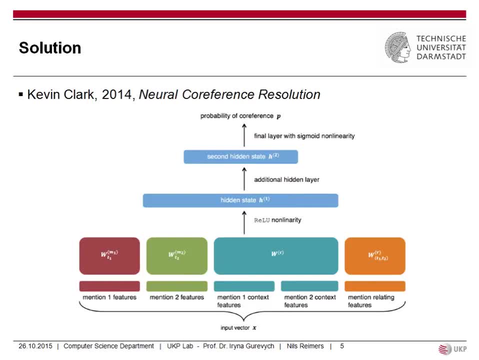 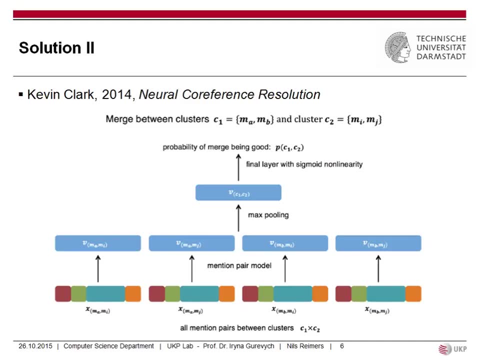 So we want to find all mentions which referring to one person and you can use like clustering, So you have like your peers and for every pair you have the information: Are they co-referring to the same person? And then he also describes a class, a merging of clustering. 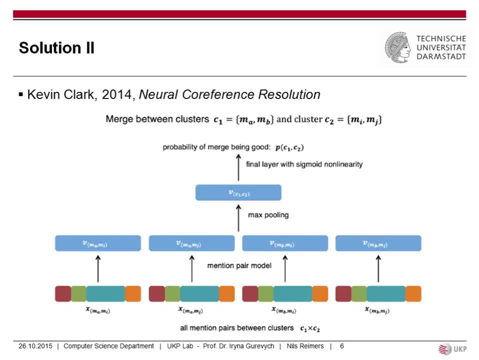 or how you can establish. should I merge two clusters? So I found one pair and another pair and are these co-referring to the same person? So should I merge the two clusters? And here he inputs every mention: in the clusters get some hidden states, some dense vector. 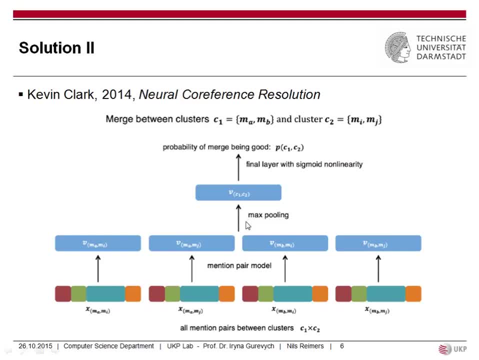 using a max pooling operation which will be introduced next week. So which looks okay. what is like the height, the highest probability over them, or the highest dense vector value, then some other hidden state and then he gets a probability of if the merge is good or not. 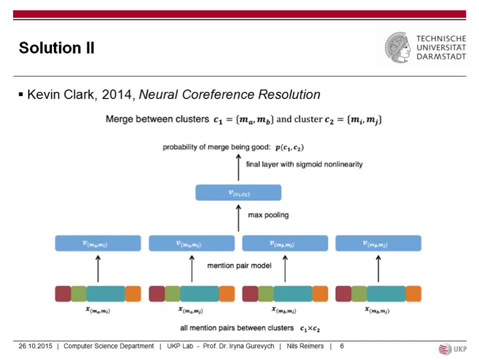 So should we merge these two clusters or is it like two different referring to two different person? And then you can use this iteratively to get from binary pairs to like your chain of co-references in that sentence, And that's how you can model your complete co-references. 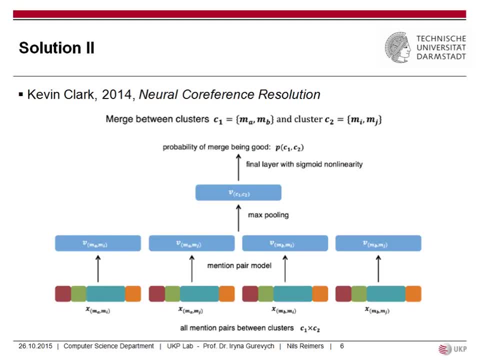 So here you have like a dense resolution system. He gets really good accuracy. It's not state of the art, but it's also not like not, So it was like class project from a student. So it's not a research, but it's really good. 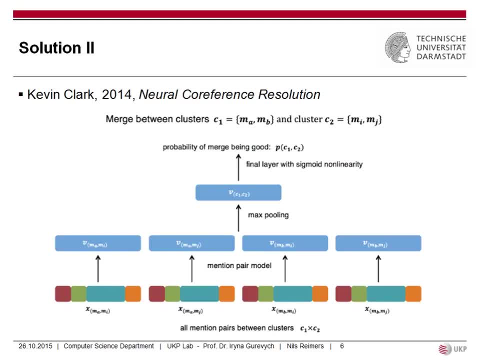 And I think I really liked the frustration on this paper. Questions on that: Can you say something to proof sentences for computing similarity? Sorry, say again. I'm saying: do you have proof sentences? You can compute also the similarity the same way. 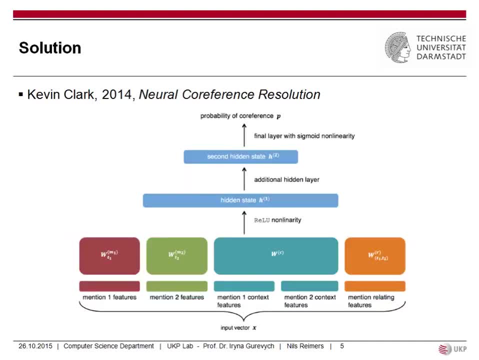 It's a question how you model like this. So how do you do the mapping from sentence to the vector space, Because sentence has a variable length, but you typically only work with fixed layers. So how you do that? we will learn one trick today: how you can work on sentences. 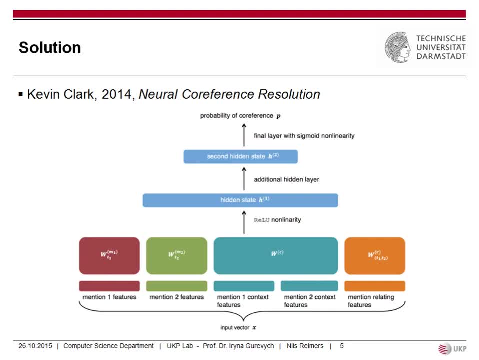 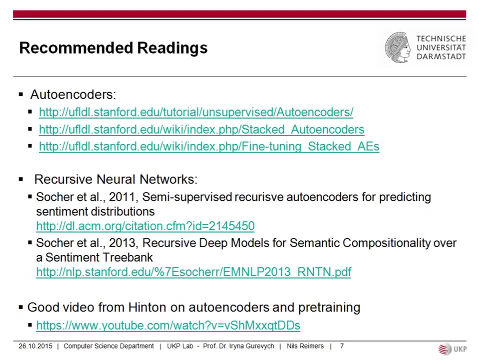 Another trick is next week on convolutional neural networks, where we can also see how we can compute it. Okay, recommended readings for today. We're going to talk about autoencoders, about recursive neural networks. So there are two papers from Richard Socher which are really nice. 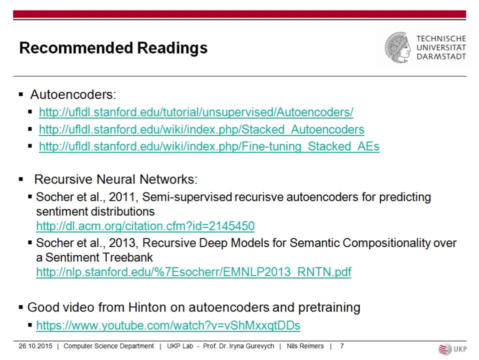 And there's a good video from Hinton on autoencoders and pre-training. So Hinton is like the grandfather of deep learning with his paper in 2006.. He started the deep learning And the video is also really interesting because he talks about sex and Al-Qaeda. 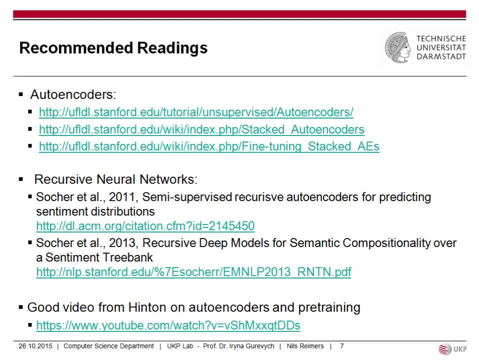 and what you can learn from sex and Al-Qaeda for deep learning and how you can map these concepts to deep learning and make your predictions better. I hope this raises your interest into watching this video, because I will not tell you what he's talking about. that in this nice video. 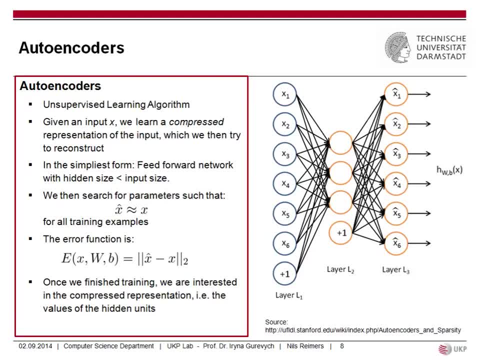 Okay, so what is an autoencoder? Autoencoder is a learning algorithm. So some people say: Some people say it's unsupervised, Some people say it's supervised, Some people say it's semi-supervised, depending how you define these words. 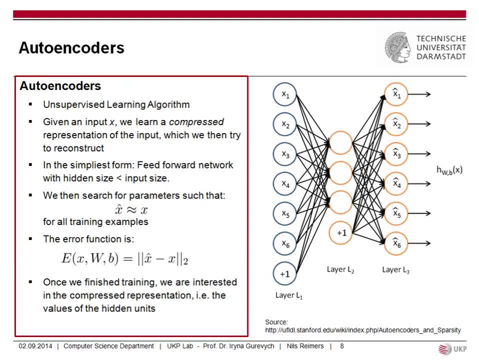 So it's a learning algorithm And it's really simple to understand and it looks really stupid in the beginning. So, given you have some input x- I don't know the pixels of your image- you pass your input, your pixels of the image, to a hidden state. 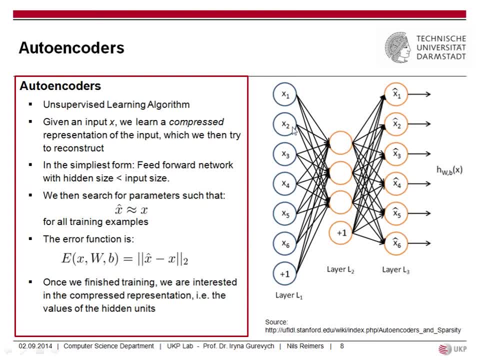 and then you try to reconstruct your input. So you have your input. Let's say you have six pixels. You reduce it to three hidden neurons And then you try to reconstruct your six pixels. The simplest form of it is a feedforward network. 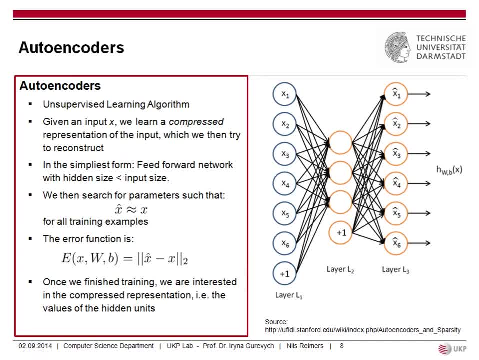 where the hidden size is smaller than the input size, And we search for parameters such that the reconstruction here is about the same as our input And the error function. we can take the mean squared error. So how big is the difference between the input and the reconstruction? 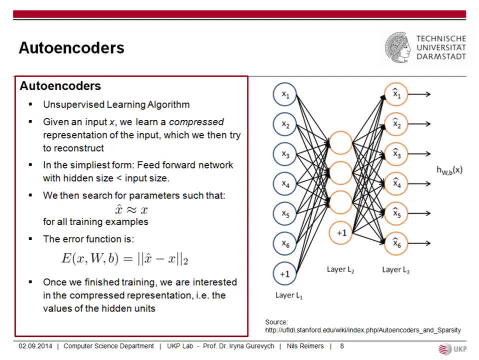 And once we're finished with training this, so you train it also with backpropagation as every other network. we're interested in this representation in the middle. So I hope it's clear how it works in principle, And now I try to explain to you why this is a smart thing and not a totally stupid thing. 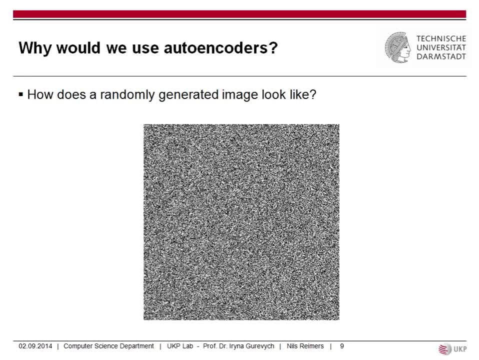 So everyone got it how it works. So the idea is you have some representation in your data. When you generate randomly an image, you get something like this: So you can generate 1 million images and there will be no real meaningful image in it. 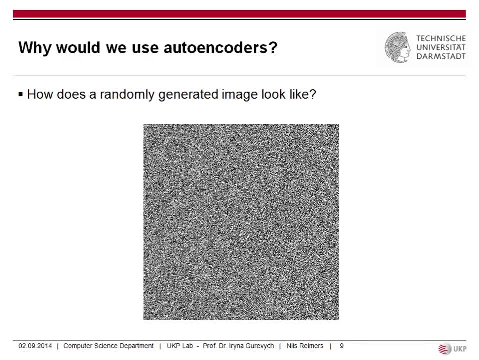 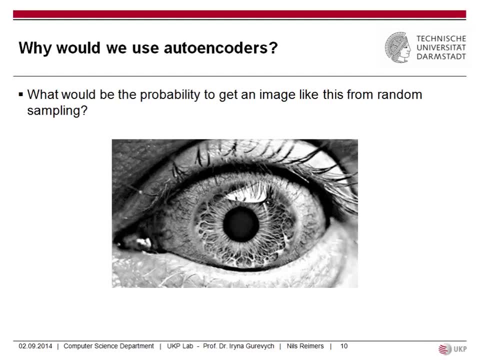 So you generate randomly 1 million images and it will all be noise. Getting an image like this is, like, really, really unlikely. The chance is maybe- I don't know- one in a trillion, So it never happens. So we have, like this, really huge space of possibilities. 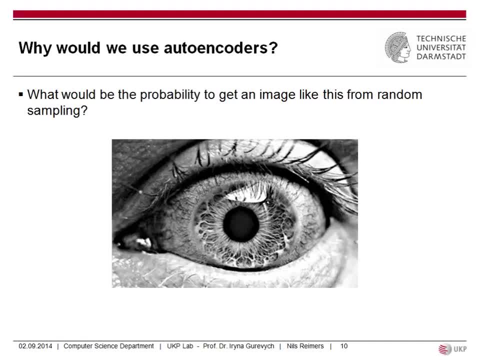 So when you think of it, this of like a dimensional space of I don't know how many pixels are there, let's say that's 40,000 pixels or 400,000 pixels, And you have a really high dimensional space. 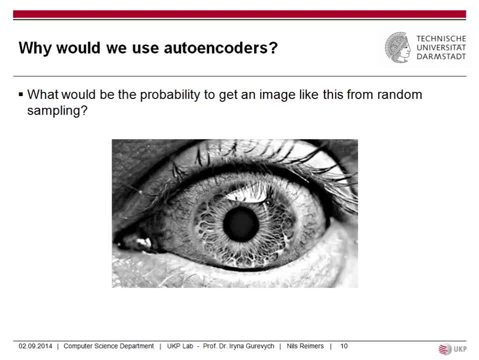 And getting some meaningful representation by this is quite rare. So what does it mean when you work on real images taken by a camera? Is that there's some hidden or latent structure in it. So, for example, we have, like soft edges, So we have patches with light, a lot of color in it, so which are dark or bright? 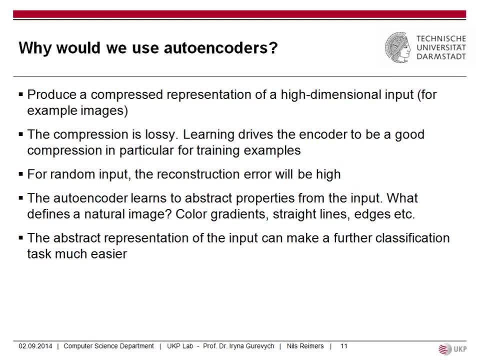 And what we do with autoencoders. we produce a compressed representation of a high dimensional input. So when you have an image of 1000 times 1000 pixels, it's like a one dimensional space. But in the one dimensional space, the number of meaningful images, the number of real images, it's like really, really small. 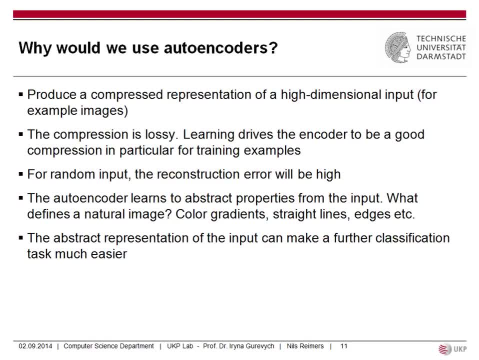 The compression is lossy So we cannot store all information in our hidden state, But we can only store some information in our hidden state And learning drives the encoder to be good compression, in particular for training examples. So when we present images, 1000 times 1000 pixels, to our learning, to our autoencoder, 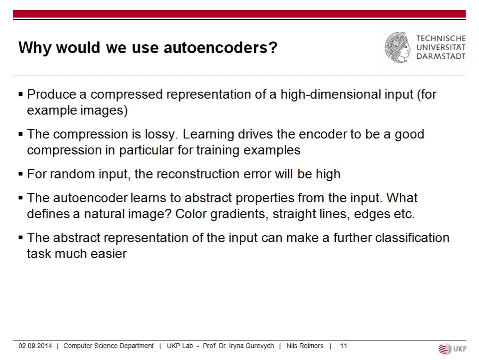 it learns: okay, what are like the structure of my images. For random input the reconstruction error will be high, But like for real images, it will be really low And the autoencoder learns to abstract properties from the input. So it learns what is the structure of like a real image. 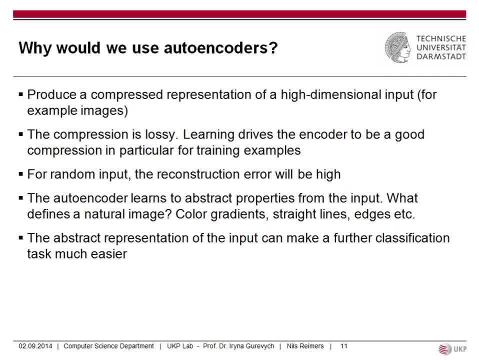 And this can make further representation, further classification much easier, because then you do not train on a one dimensional space, But you train maybe only on a 100 dimensional space. So when you reduce the 1 million input pixels to 100 hidden state, 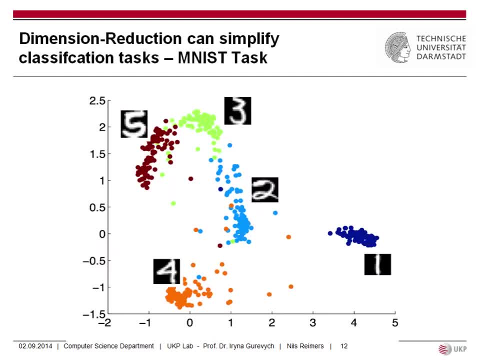 this makes classification a lot easier. So one example is on the MNIST example, And here they trained it. on the pixels, It's only 784, 886 dimension input. reduce it to two dimensions And we see that similar numbers, pixels, the pixels of similar, are close in the space. 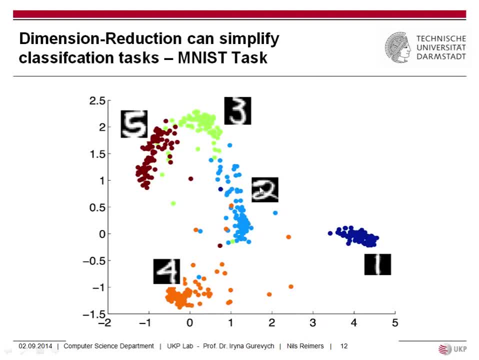 So here we see all the fives, here we see all the ones, here we see all the twos. And now drawing like classifying or classify these images into classes, which is really simple for a human. You could just draw some lines and get quite okay accuracy on image recognition. 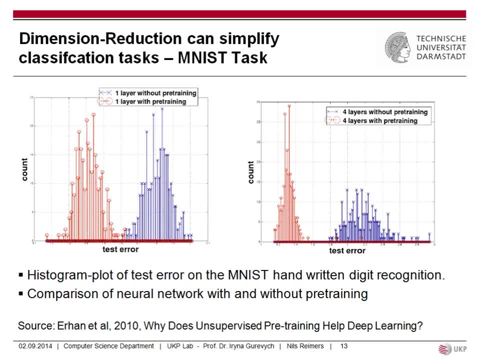 You can also put it in more like scientific way and scientific measuring. There's a really nice paper- why does unsupervised pre-training help deep learning- which is a really good read on it. What he did is he tested the MNIST handwritten digit, that data set computed, error, error. 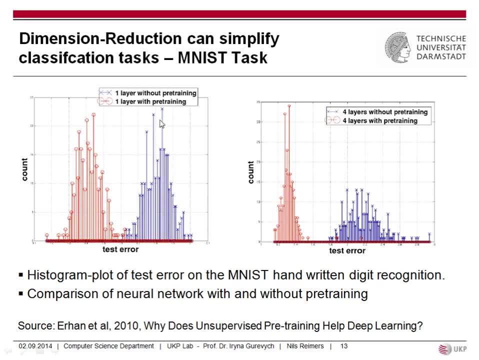 So here we see, it was one hidden layer and he has without pre-training. So pre-training, I will come in a moment. So pre-training is applying autoencoders first to input the image of the handwritten digit and then try to reconstruct and then use this as a first step. 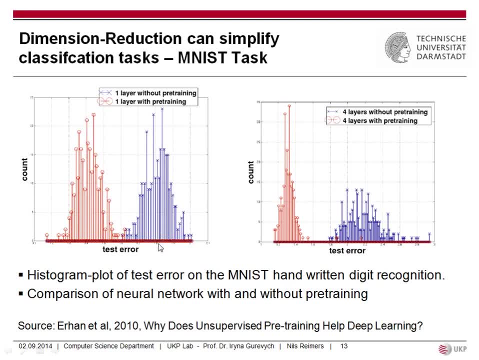 And you see, without pre-training, the error rate is very low. And you see, without pre-training, the error rate is very low. And you see, without pre-training, the error rate is very low. The error rate is around here, so it's 1.3.. 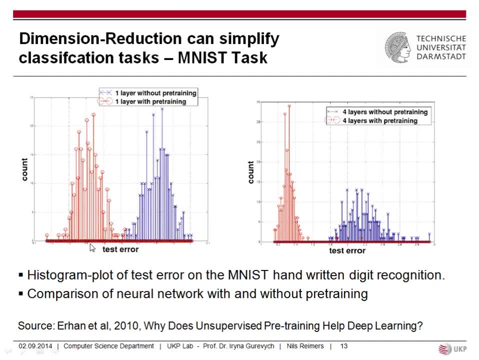 And here it's like lower. it's this like 2.. So this is lower error rate. error rate of 0.. And pre-training helps And you have this especially in deep neural networks. So when you do not apply pre-training in a deep neural network, you get like really high error rate and also an error rate. 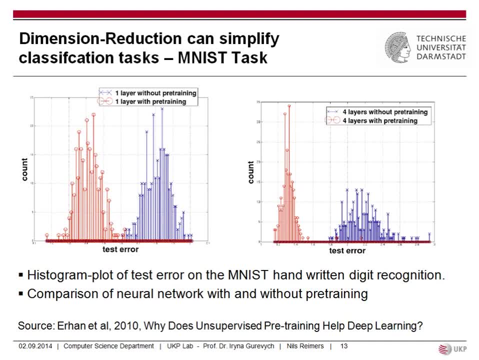 which is not superior to like in a network with only a single layer. But when you apply pre-training With autoencoders, you can decrease the error rate, And that's also what Hinton presented in his 2006 papers. He applied for the first time pre-training with autoencoders, a kind of autoencoders. 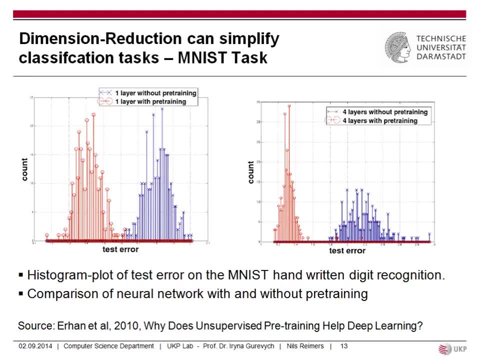 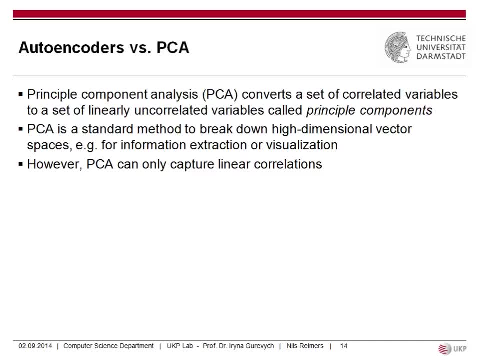 And this was like the crucial breakthrough in deep learning and learning training- deep neural networks, So autoencoders- is kind of similar to PCA, principal component analysis or LSA. So in PCA, In PCA, we convert a set of correlated variables to the principal components. 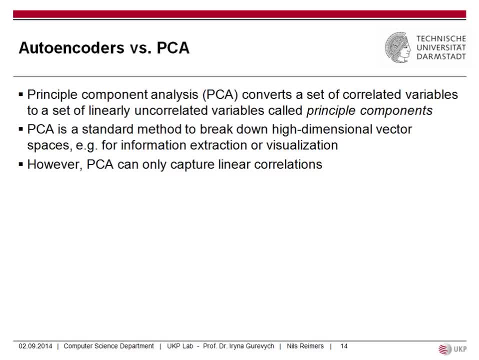 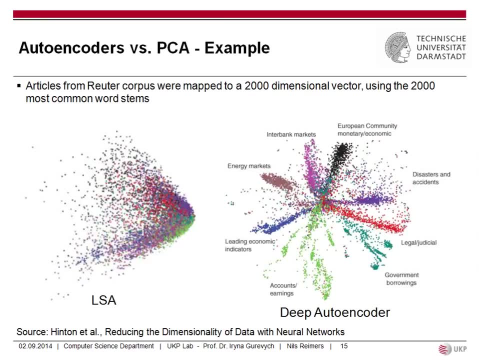 The problem with PCA: it can only capture linear correlations, So any nonlinear relations in your data cannot be captured with PCAs, And What Hinton does show in his presentation. So So he took the Reuters corpus of news articles and reduced it to, or used the most common terms in it and reduced it. 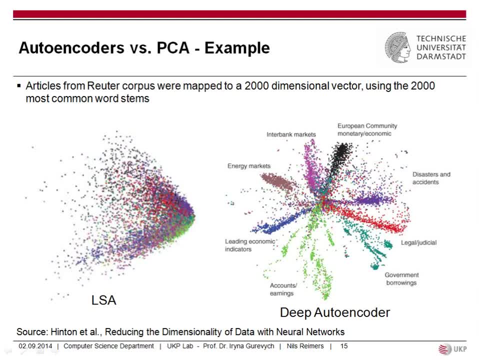 And with LSA we get an output like this. But when he applied also a deep autoencoder and he got an output like this. So here we can see all accounts or earnings articles. Here we have articles on energy market, Here we have like legal documents, which gives us a really nice clustering of similar documents. 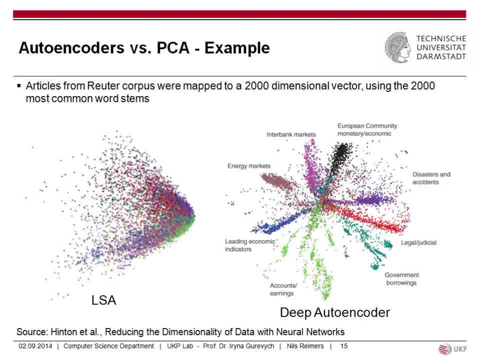 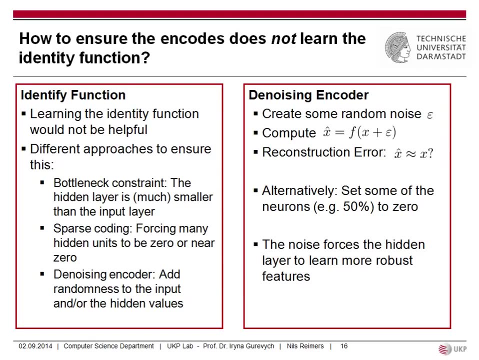 Because in a document you have really a lot of non-linear correlations in it. Any questions on that? So I hope we all agree that autoencoders could be good And The question is: how do we ensure that the autoencoder is not learning the identity function? 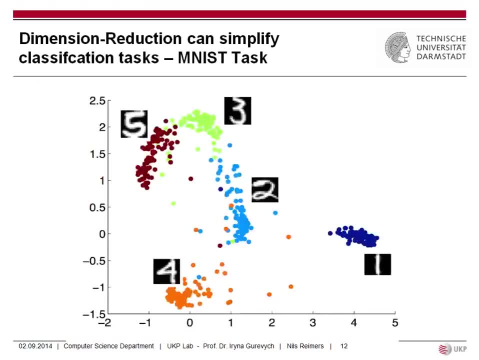 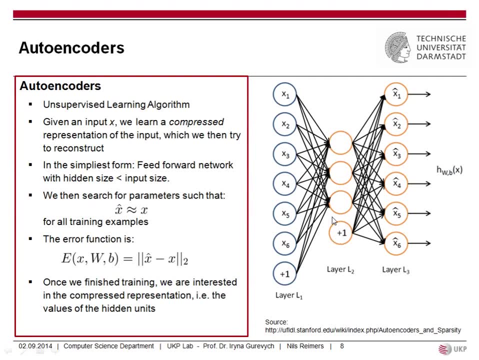 So learning the identity function would not be helpful. So In our example, if we just put six hidden layers here, the reconstruction would be really easy. So the first neuron would learn the value of the first input, The second neuron would learn the value of the second input, and then we get like zero reconstruction. 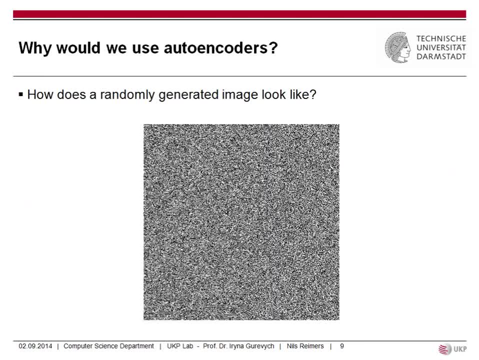 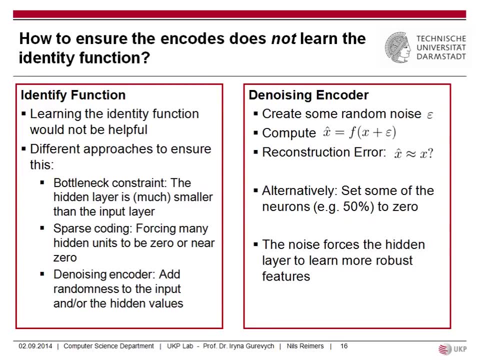 But learning the identity function is nothing really helpful. So there are different ways how you can avoid this. The first one is the bottleneck constraint, So the hidden layers. The hidden layer is much smaller than the input layer, so you have like one million pixels as input and you constrain it to like 1,000 hidden layers, so it needs to reduce from one million input to 1,000. 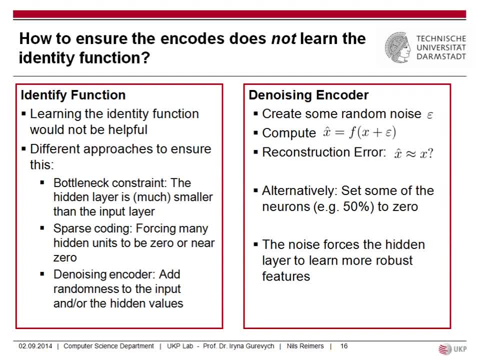 Then there's the sparse encoding, where you force many hidden units to be zero or near zero, And there's the denoising encoder. so you add randomness to the input and or to the hidden values. So there's the denoising encoder. 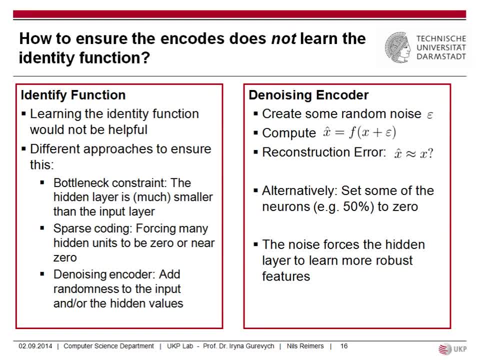 So there's the denoising encoder, so you add randomness to the input and or to the hidden values. And there's the denoising encoder, So you create some random noise and the random noise is added to every neuron and then you try to reconstruct this error. 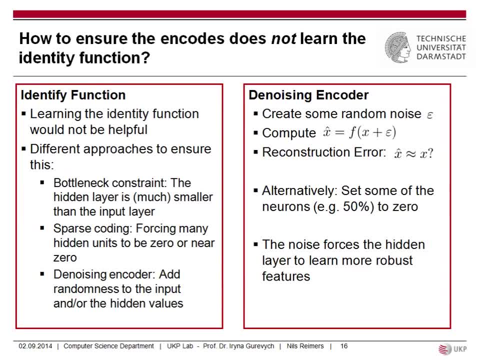 Alternative implementation is that you just dump, for example, 50% of the hidden states. So you do your encoder, go from the input to the hidden state and then you just delete 50% of the hidden and then it must be reconstructed from like only half of the hidden states. 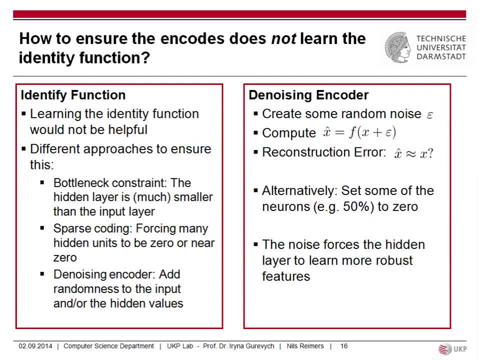 Is it like a dribble? It's a dropout layer, So this one is really easy to implement. bottleneck constraint, The dropout layer, or denoising encoder, is kind of similar to a dropout layer. Dropout layer where you delete 50% of the hidden states, is really cool. 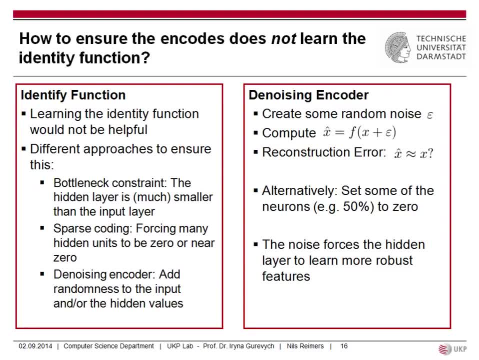 I was totally amazed when I read on this on Friday or Thursday And I will explain you the math later in the third part of this lecture Why it's really really cool. It's a really interesting concept And the most people use like a dropout layer for autoencoders. 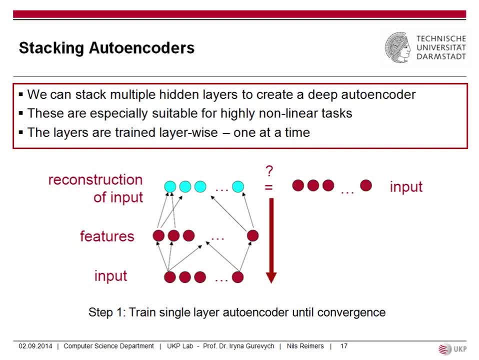 What we can also do is like to stack autoencoders. So we start with, like our input, our first hidden layer, and then we try to reconstruct the input And we can this, of course, stack for several times And we will run it layer-wise. 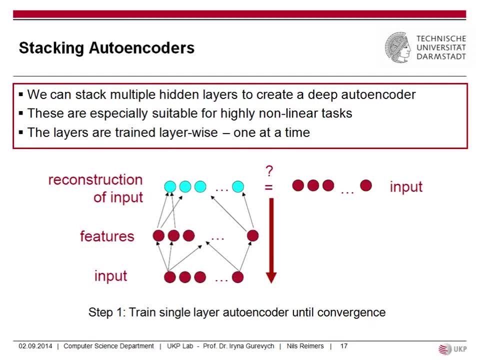 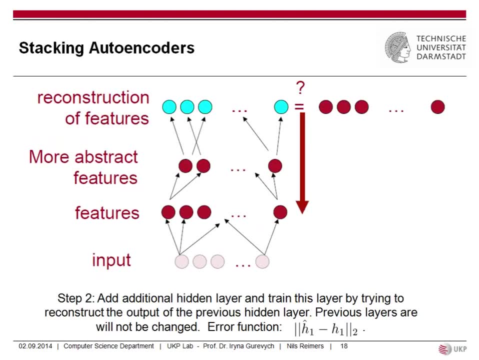 So we start with, like our input, our first hidden layer And then the reconstruction of the input. We train it until we're satisfied with the results And then we go on. We say we keep our hidden state, this fixed, And input it as an input to the next autoencoder. 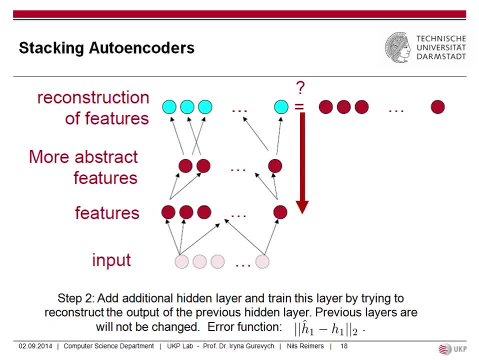 So here we have more abstract features, representations, And we try to reconstruct it, And this is how we can stack arbitrarily many documents. So in the second step we try to compute the reconstruction, The reconstruction error, between our predicted hidden value 1 and the actual hidden value 1.. 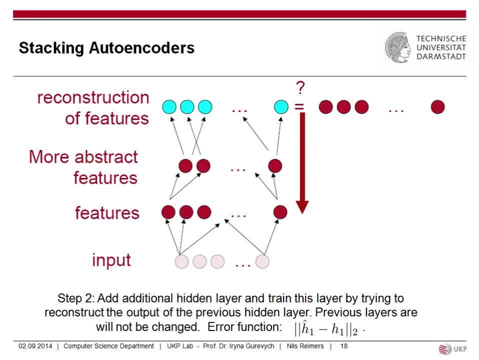 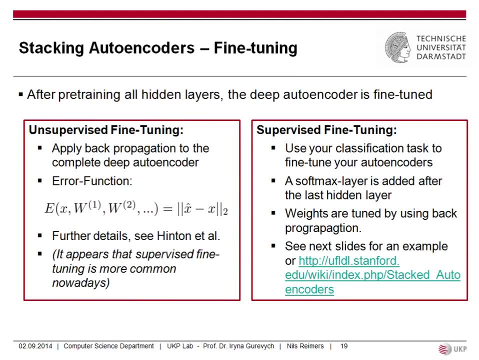 And this is how we can train arbitrarily deep neural networks with autoencoders. After that you do some fine-tuning. So when you train every layer of your hidden layers, you do some fine-tuning So you can apply the backpropagation to the complete deep autoencoder. 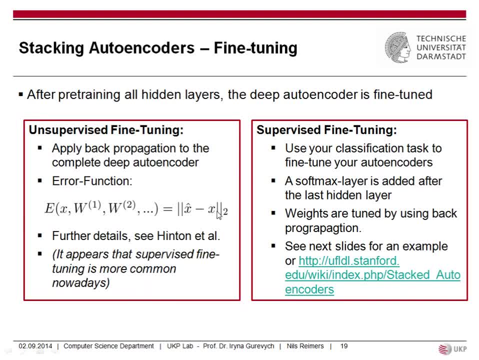 Where you input your Value and try to reconstruct. So, for example, you have three encoders Making the hidden layers smaller and smaller and smaller, And then you try to reconstruct it, Or you can do some fine-tuning So you have a classification task. 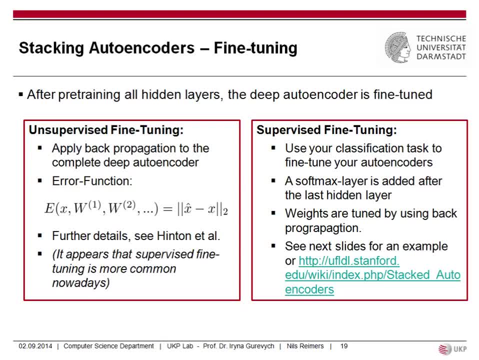 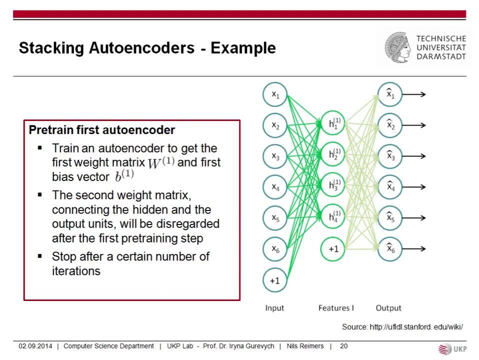 For example, the label for your images of the digits, And you just apply a softmax layer as the last layer And then you do normal supervised training on that. So to give you an example, we start with six inputs, We reduce it to four hidden layers. 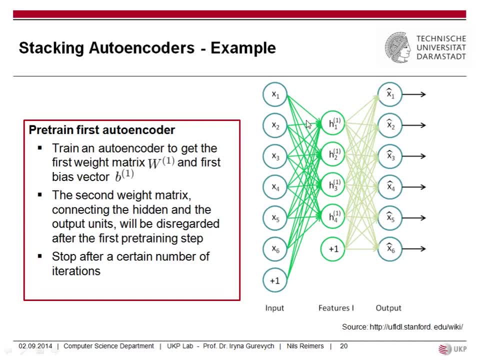 And you train an autoencoder to get the first weight, So to get this weight matrix and the first bias vector, So which is like depicted here. And then you try to reconstruct it And after a certain number of steps, iterations, you stop. 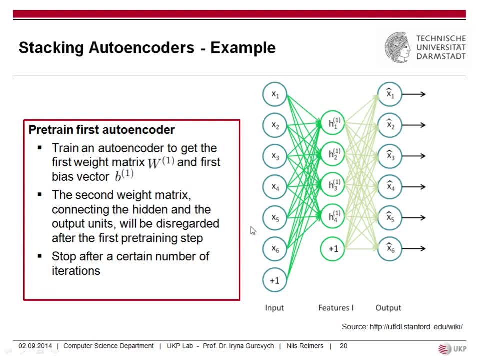 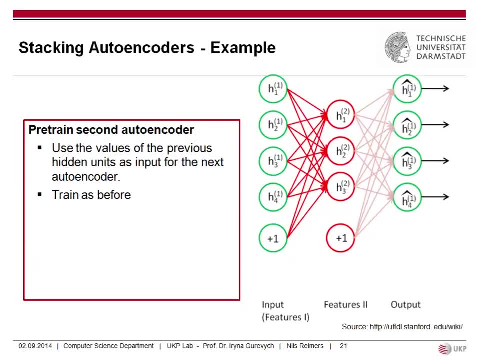 You neglect this information. this decoder- here This is called the first part- is the encoder, This is the decoder, And you just dump it. So what kind of function is in the output layer? Do you like tangential supercubicles or some standard ones? 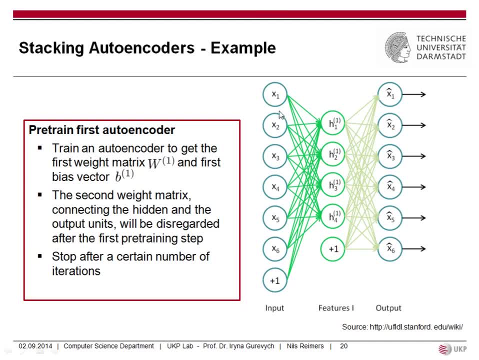 Yeah, So it usually depends what. How is your values encoded? But you can use tangential supercubicles, But the output of it can only be between minus one. So when you put I don't know 10,000 in here, 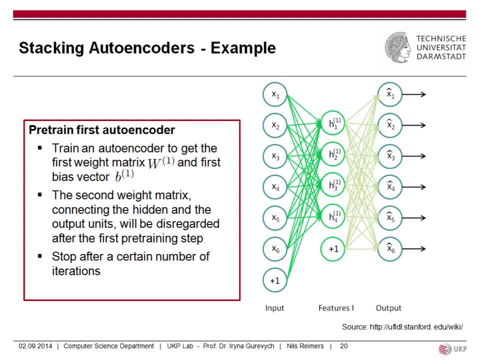 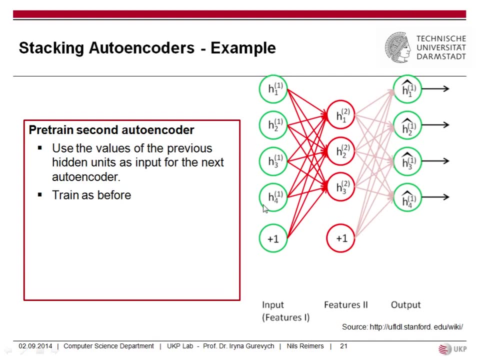 You cannot reconstruct it in a meaningful way. So, when the input should also be between minus one and one or between zero and one, Good question. And after some time you're happy with the results. So you start a new autoencoder. Take your output for the first hidden state. 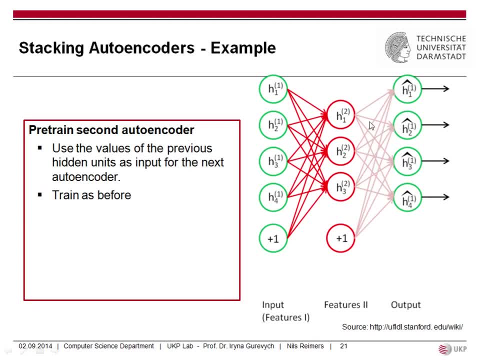 Train the weight matrixes here, Try to reconstruct it, Train it as before, And after some iterations you said: okay, my loss function is small enough, I will converge to the next layer. And then you can say: okay, now you have the hidden layer two. 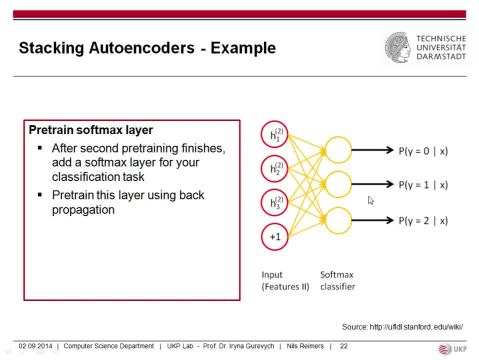 And you train your self-max classifier And you compute. okay, here you have three classes: Class zero, class one, class two, And you can try and pre-train the softmax layer And then you can do the fine tuning. So you start with your actual input. 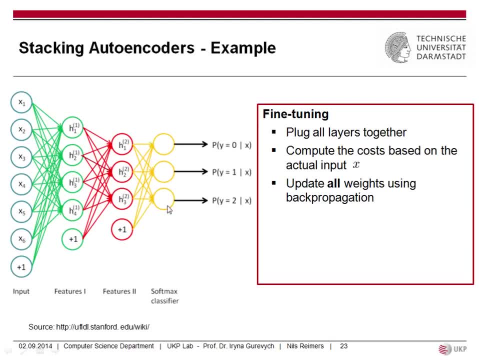 Map it to the first, Map it to the second hidden layer, Map it to the softmax classifier And then do back propagation over all the input Questions. So the whole idea is here, that you set up the So for learning end-to-end. you have better weights for the neurons. 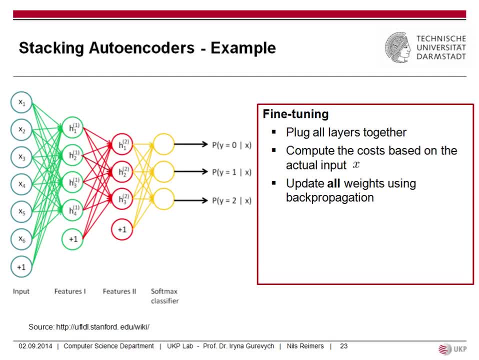 Is that important For the population? Correct? So does it make a huge difference? We will come to it on the next slide. If it makes a huge difference, it sounds very complicated And it's really annoying to implement, Because here you have one first training, second training, third training. 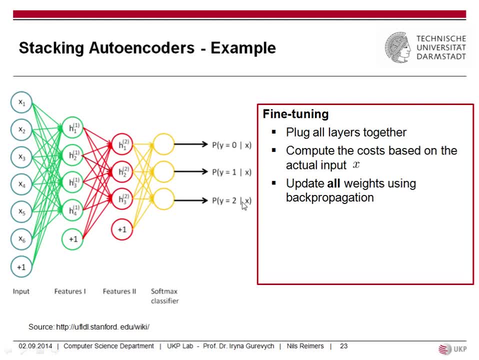 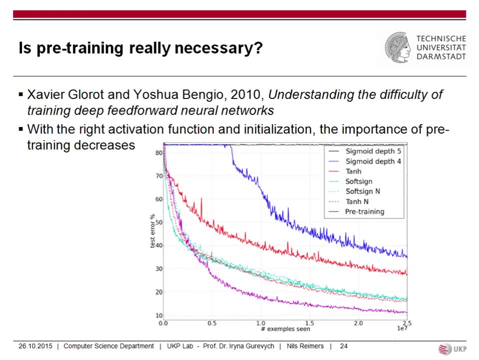 And then the complete is the fourth training. So you have four training iterations And you need to see, okay, how many iterations do I need, And take some time. So how important is it And is pre-training really necessary? So Hinton presented in his 2006 paper the idea of pre-training. 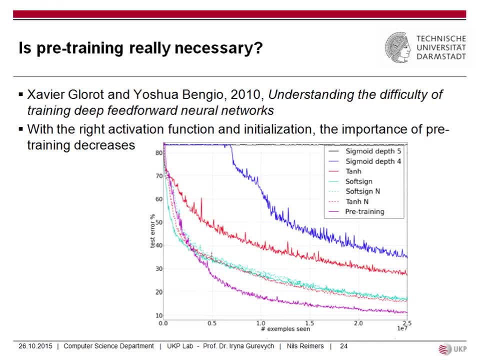 which was like the breakthrough in deep learning, And Gloroth and Bengio presented in 2010 in the paper Understanding the Difficulty of Training Deep Feedforward Neural Networks, a different internalization function and different activation function. So you see maybe in Keras how we can initialize a dense layer. 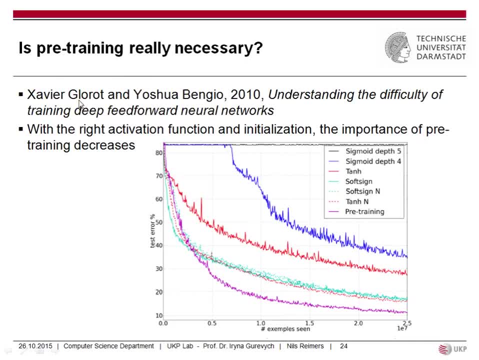 with like, using the Gloroth function which was presented here in their paper, And they worked also on the MNIST handwritten digit data set at training different networks. So here up here we see sigmoid with depth five. So they use five hidden layers and use the sigmoid function. 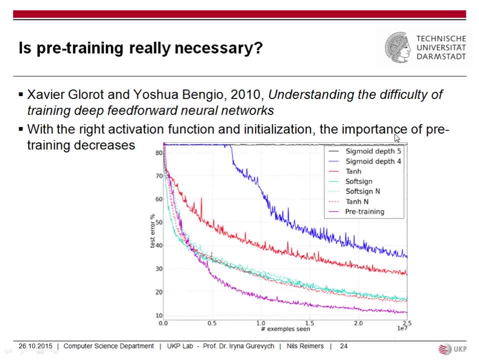 and it's not learning anything. So sigmoid function is really bad. It was also discovered In their paper that sigmoid function is really bad And you should use the tangent-globulical function because the mean value of the sigmoid is 0.5.. 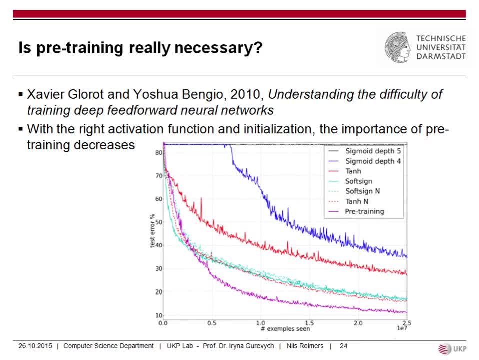 The mean value of the tangent function is zero, which is much nicer. When you use the sigmoid function with depth four, you have really high error rate, and then it starts slowly to decrease When you just change the activation function to the tangent function. 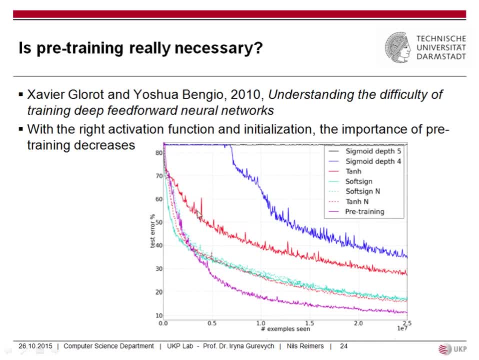 it's not changing anything else. You get a really good or get a lot better or a lot lower error rate on that. Then he also did some soft sign function which is similar to the tangent function but it's a bit easier to compute. 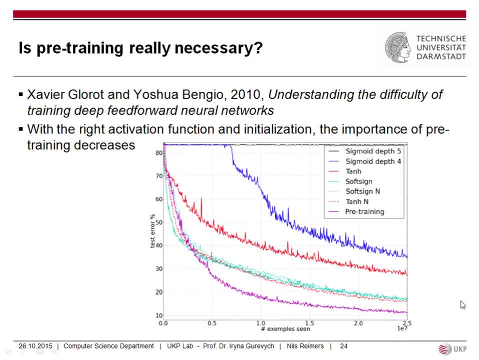 It's not really used, I would say it's not really common. but then he presented different normalization methods, So he presented a new way how to use it, how to initialize the weights, which is called here n, And we see, okay, when you use the tangent function. 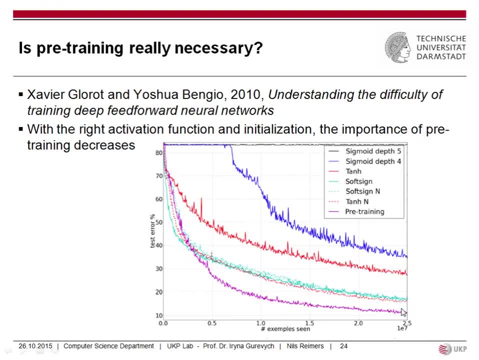 with the right normalization you get quite a low error rate. Oh sorry, it's not on the MNIST data set, it's on a different data set And you get quite a low error rate when you compare it. So here you have like an error rate of 15%. 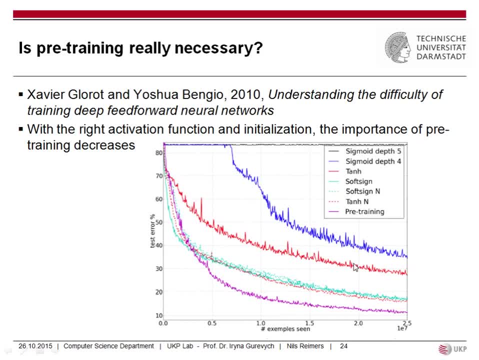 compared to 90% when you use the sigmoid function. But it's still a bit higher than with the pre-training. But with the right activation, function and normalization the importance of pre-training decreases And I think in the most recent papers you usually people do not apply pre-training that much. 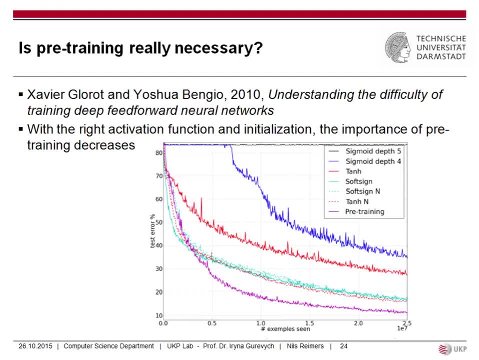 Yes, So if I understand that correctly, if I follow this way of constructing the network, then the layers always get smaller, right? Because otherwise I'm running this bottleneck problem. So yeah, you want to run, so you can either run. 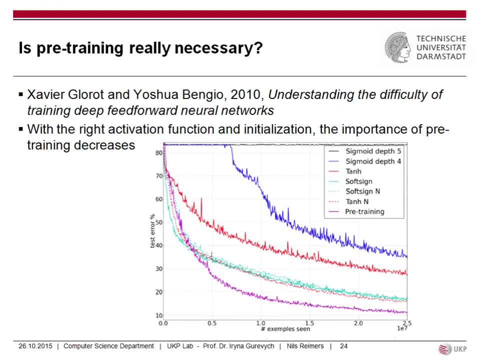 you want to make them smaller, to have the bottleneck problem. So you want to force the network that it's not doing the easy job and learning the identity function, but it learns the relations. what are the important relations in my data? But is that really common? 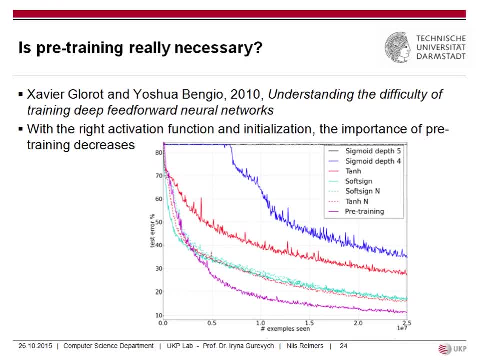 that all the layers get smaller towards the end, or It's really common to do this, yeah, So basically you start with a big layer and then it gets smaller so that you can learn more abstract information on that, more abstract representation of your data. 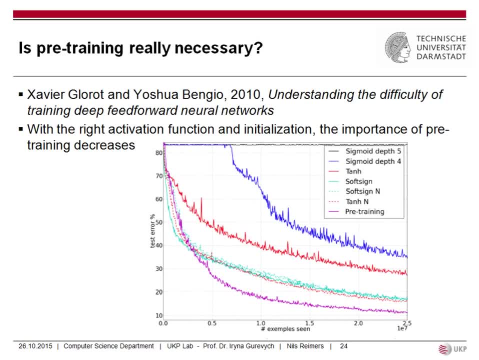 So you start with really simple for the computer vision, for example, taking edges in your data, and then some in a really deep layer. you can detect whole faces, or you can detect cats, or you can detect cars. That was exactly what I was wondering. 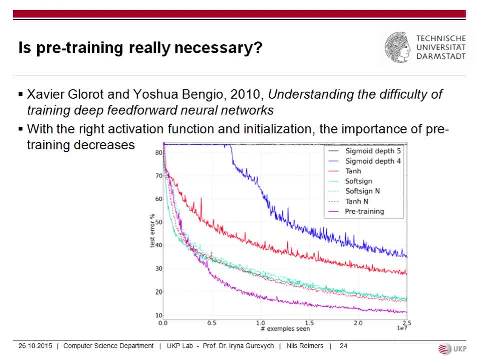 because if I have one layer- and I have- which detects edges, There are not so many combinations of edges. I mean there are edges like that, edges like that and all that stuff, but there are not so many. But when it comes to more complex structures, 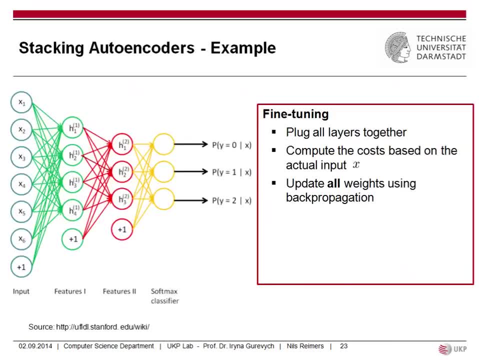 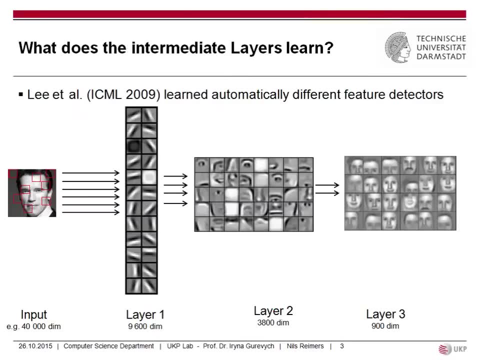 like eyes and ears and something like that, then I think it would make sense to have a bigger layer of these. So in computer vision they use something which is called convolutional neural networks, which is covered next week. So you start typically on a really small patch. 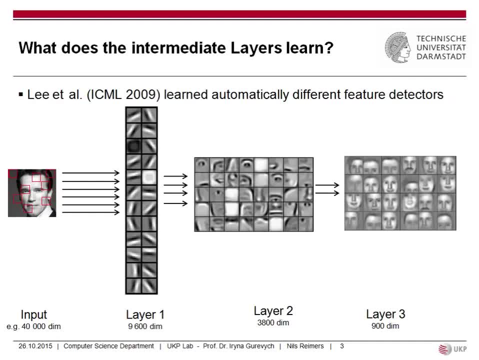 so like, for example, 9 times 9 pixels, and you scan with the patch over it and this gives you then some, for example, 9,000- dimensions for the different patches. So you have only small input: 9 times 9 pixels. 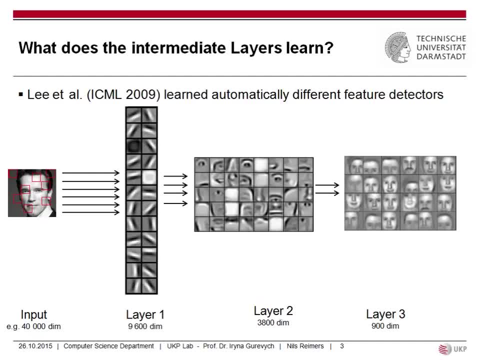 but because you have so many different patches, the hidden layer gets bigger And then you combine different patches. so you take, for example, you increase it, you go from 9 to 9,000, you go to 9 pixels, you go to 3 times 3 patches. 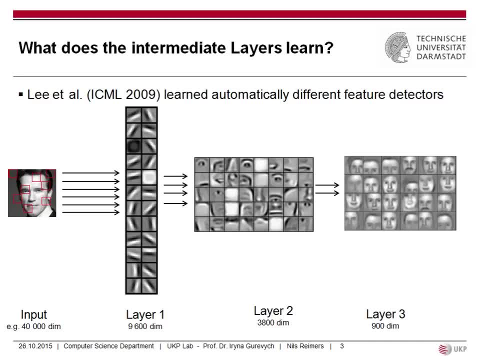 so it starts to be 27 times 27 pixels And then you get something like this and then you combine these patches again to something bigger and then you get one final output out of it. But when you combine the number of patches, 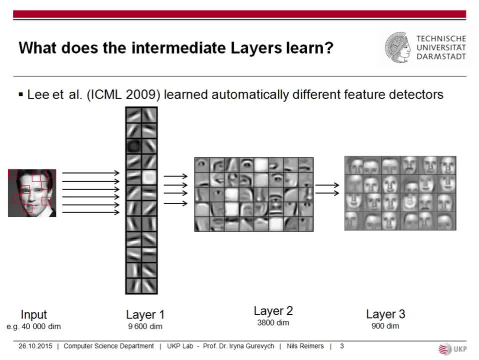 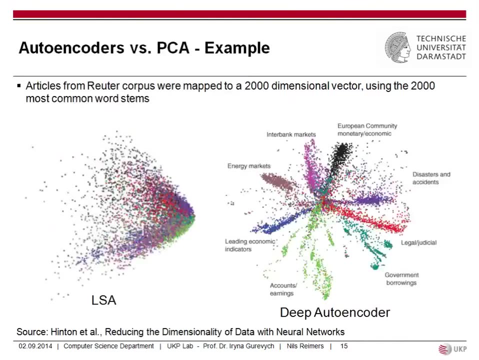 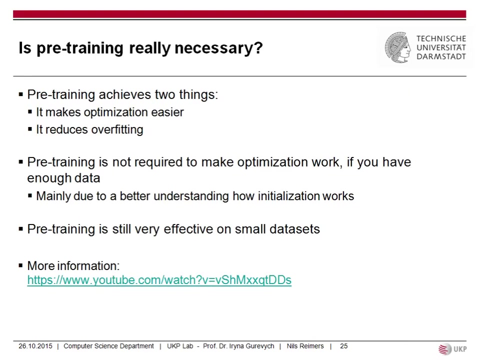 so the input gets smaller for everyone. so here it's the smallest, at the end it's the biggest, but the number of suitable things or suitable formations is quite small. So pre-training achieves two things: It makes optimization easier. so when you have a really deep network, 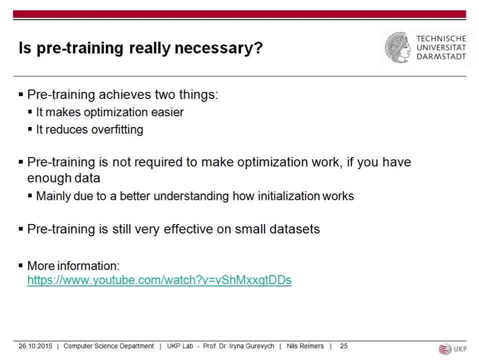 you have the problem that when you compute the gradient that the gradient vanishes. When you have a deep network- So let's say you have depth five- then one link in the beginning, so one weight in the beginning did not really make any difference for the output. 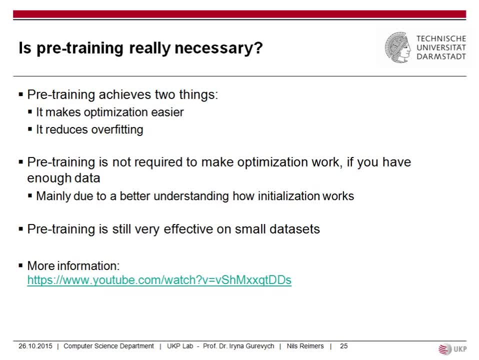 and your network is not learning anything and it also reduces overfitting. Pre-training is not required to make optimization work. if you have enough data, so mainly due to a better understanding how internalization works. So when you read older papers, they are all about pre-training. 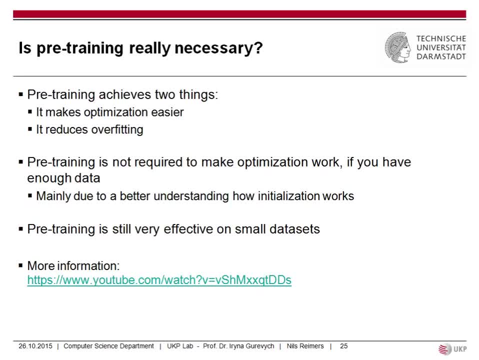 and then people focus more on how. why is not super-wise training not working? But pre-training is claimed to be still really effective on small data sets, And if you want to have more information, there's another YouTube video where I think Hinton again talks on that. 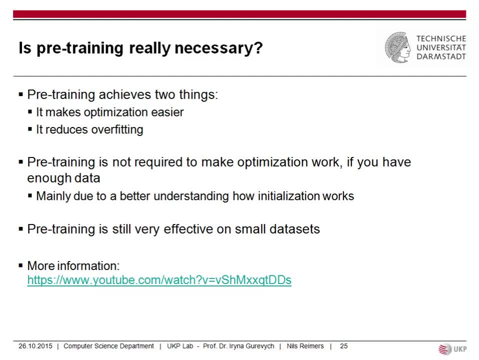 so what is pre-training? when to use it? When you have large data sets, you don't need to do it. Okay, this is so much on autoencoders and pre-training Questions on that on the theory side. So to the small data set. 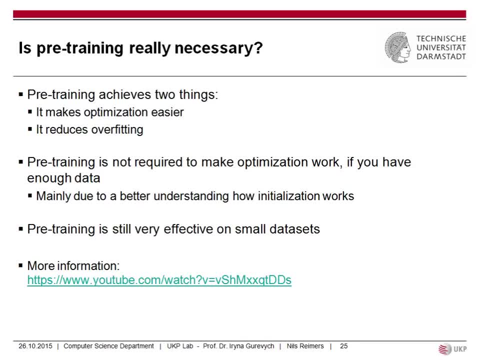 I mean usually in a situation where you have a small data set labeled and then you have large data set unlabeled. so it would make sense then if you pre-set up your hidden layers on the unlabeled and then train a model on the labeled. is that right? 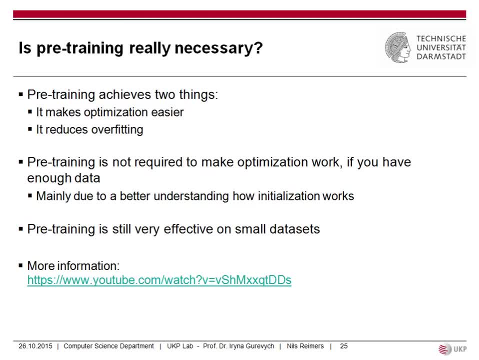 Correct. I mean it's similar to do what we do with word embeddings. So word embeddings are kind of similar to autoencoders. So you have a word or a context and you try to predict the word, or you have a word and try to predict the context. 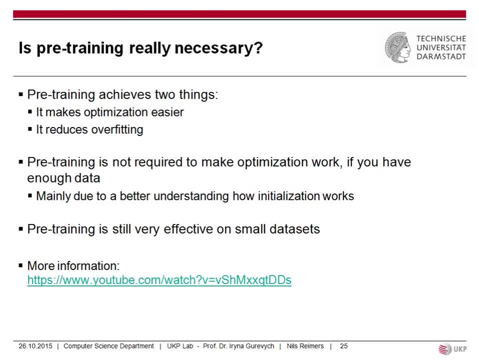 in the script-gram model, which is also working on unlabeled data, And this can significantly boost your network. But when you use word embeddings as first layer, I would not recommend that you go into the hassle with pre-training your network. Let me try that for you. 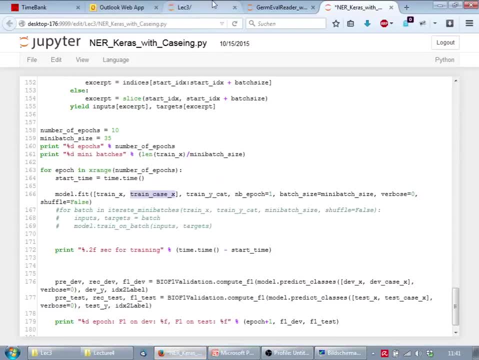 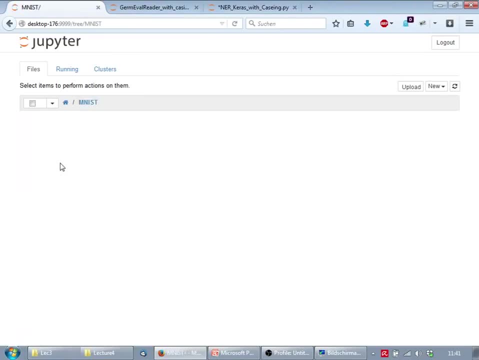 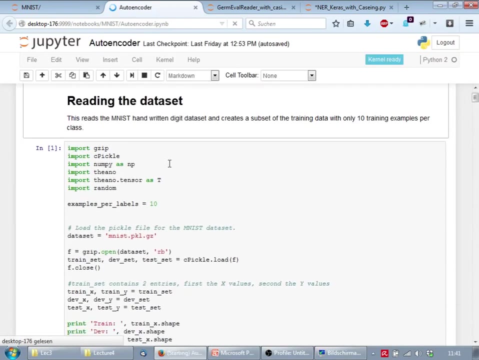 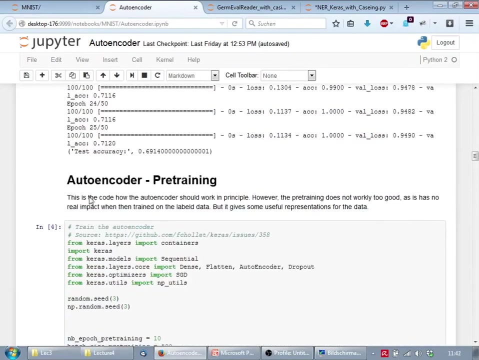 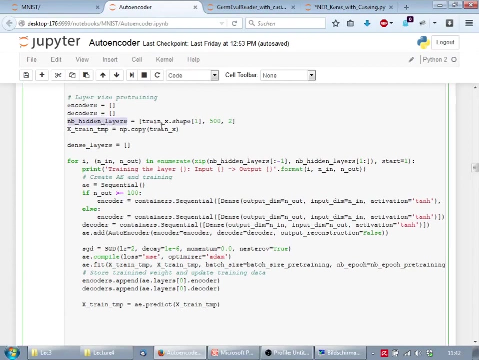 Yeah, I tried it. There's awesome implementation in the GitHub. So, on MNIST, I tried to implement it and I failed, so it does not produce better results. Let me check. So how does it look in principle? So here we can define the hidden layers. 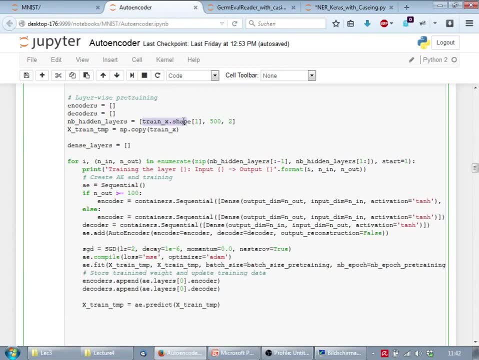 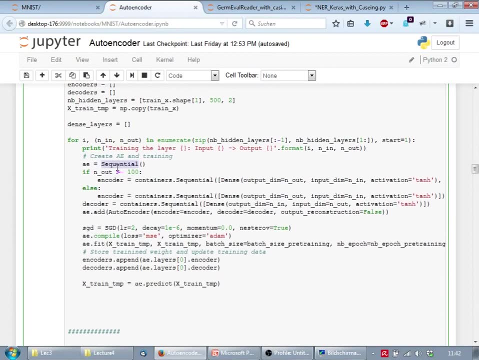 So we say, start with like the size of it, and then we go to 500, and then we go to two dimensional And we do it by defining a sequential model And we have an encoder where we use the dense function with activation function, the tangents. 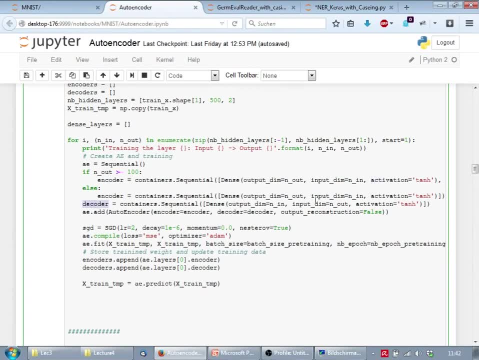 And we have a decoder, where here output and input domains are flipped, So we go from 700, 84 to 500, and then for the decoder from 500 to 700, 84.. And then there's an autoencoder function in Keras. 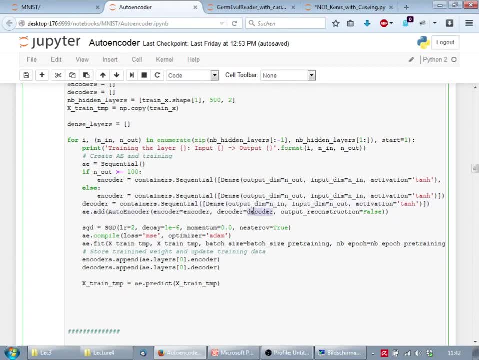 where we say: okay, we have an autoencoder. We say: we have an encoder, we have a decoder, We can define our optimizer either as the gradient descent or the atom function, And then we train or call fit to train the model. 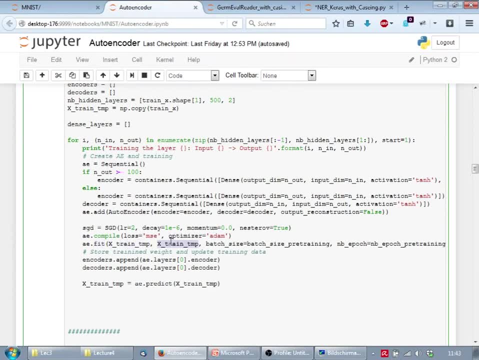 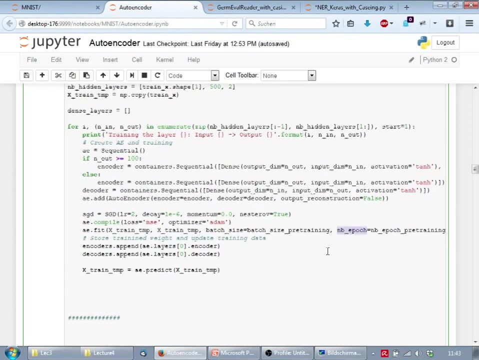 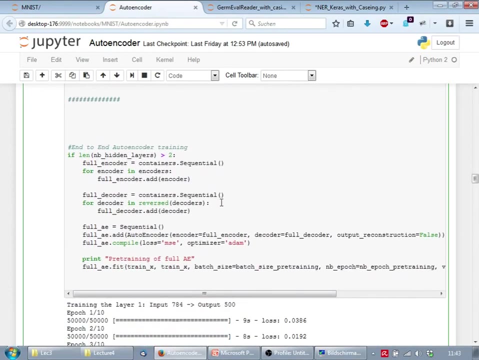 So we give our input as an X, our output, our label, which is also the X matrix. We have some batch size, We have some number of iterations and we do it in an iterative way. So train layer by layer, And then we can also do an end-to-end autoencoder training. 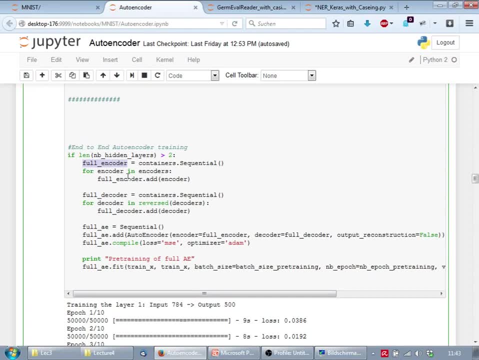 So for our encoder, for every encoder, we have matrix with all the encoders. We add all the encoder to our model and then we go in a reversed order with decoders: add all decoders. We add all decoders to our sequential model. 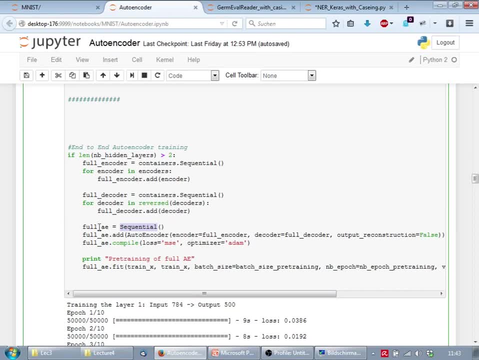 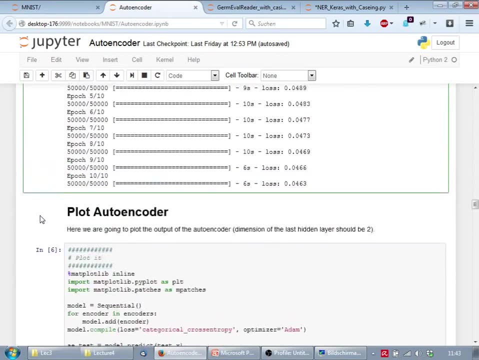 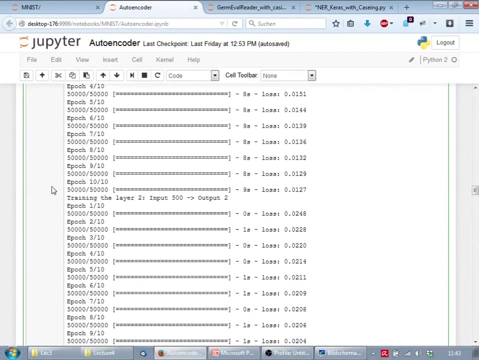 And then we train our full autoencoder end-to-end, And we can do that. And here I have the run plot. There was okay, I didn't run this again or I'm not on the latest version, but it gives you like nice plot of X. 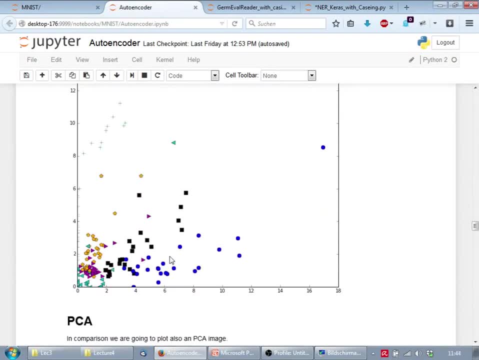 where you can okay some distinction between the different layers. So here I used a different activation function, which gives you a not really bad plot. If you run it with, I think, tangents function, it gives you a much nicer plot. 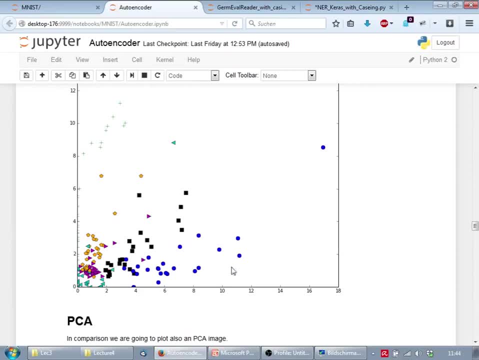 So this is on a rectifier linear unit. It's not really not looking so good on a rectifier linear unit. When you use it on the tangent function it gives you a nice plot where you can see the difference in it. It does not really help for the classification task. 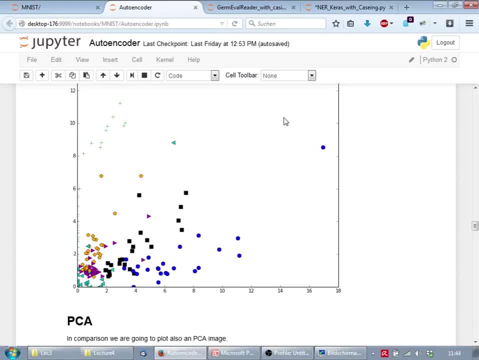 in this setup. So there's somewhere a bug. It's maybe not converging. not enough iterations, batch size too big, too small, I don't know. If someone figures out, please inform me when you say: okay, you forgot to do this step. 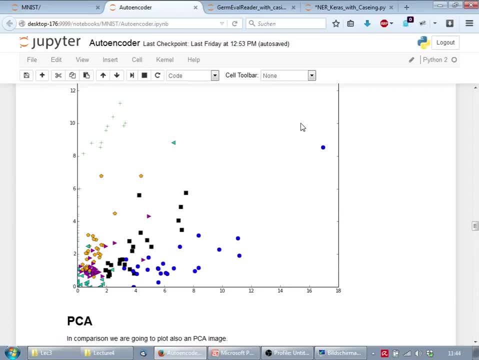 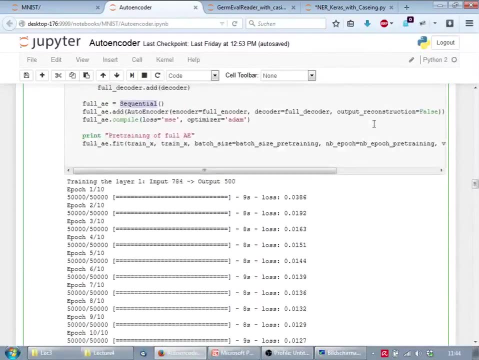 Just shoot me an email. So I'm really interested in. but that's in principle how you train your autoencoder for it. So it's some mess in the code, but it's still quite easy. So you define your encoder, your decoder. 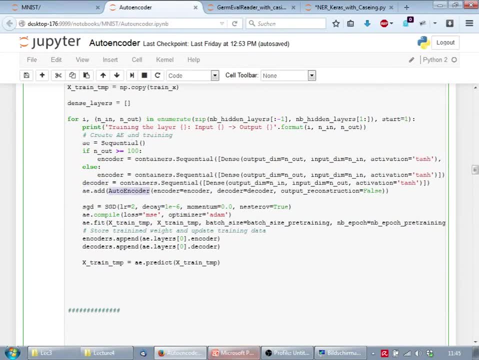 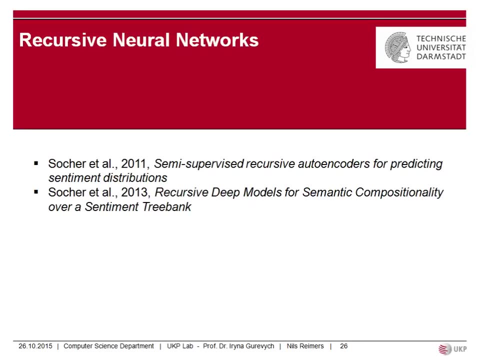 find your autoencoder and just train it. Okay, Next, So why do we care about autoencoders? So there's, as mentioned, what we a lot often do is that we have not fixed sized input. So when we do sentence classification, 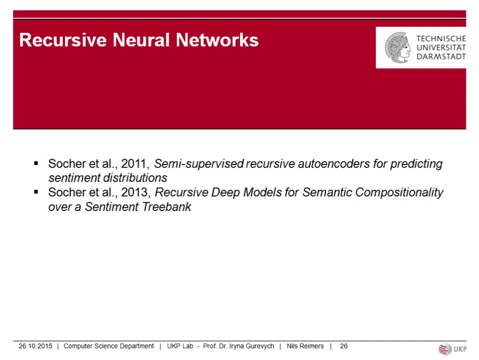 or when we document classification, it can be variable in length. And how to deal with the variable length? there are two approaches. One is convolutional approach, The other one, well, three approaches, And the first one is recursive neural networks. 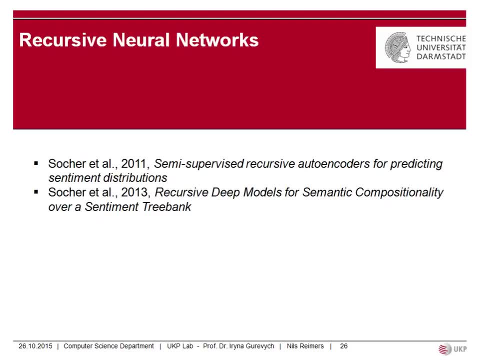 which will be covered this week And in the next two weeks. we will cover the two other approaches And there are two papers by Zofar: semi supervised recursive autoencoders for protecting sentiment distribution and recursive deep models for semantic conversionality over sentiment tree bank. 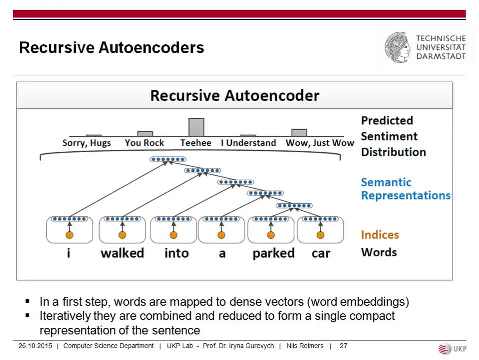 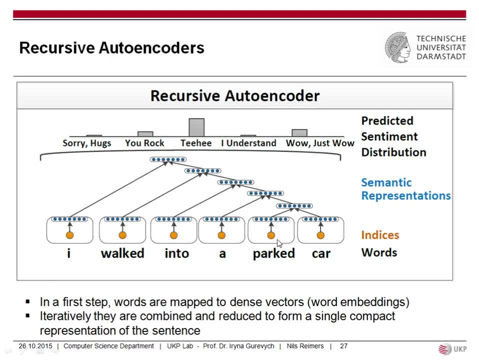 So here we have, is this a recursive encoder? And so in this case, in this sentence, I walked into a parked car And we have our word embeddings, where we can map every word to some word embeddings to some dense vector. And in his 2011 paper, 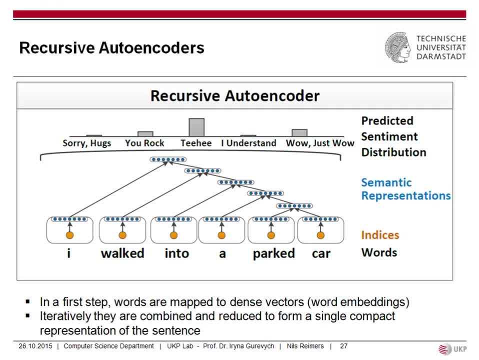 he took two words and combined these word embeddings to a single word: embedding. So let's say we have 100 dimensional word embeddings and every word is mapped to 100 dimension vector. then you take 200 dimensions as input and map it to one single 100-dimensional vector. 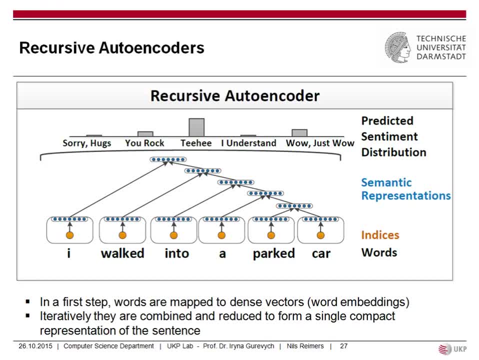 How could you do that? Any ideas how you could map 200 dimensions, two vectors of 100 dimensions, into one vector of 100 dimensions? Yeah, PCA would be hard. PCA would be hard. What we could do is just add them. So you add two or you do take the average. 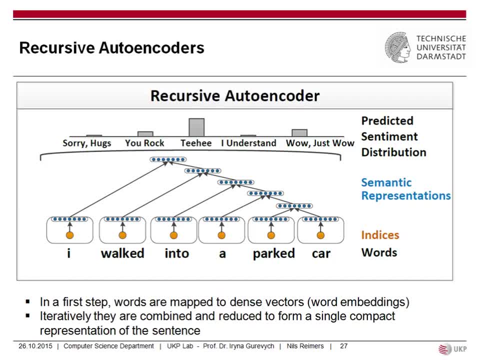 No solution, No solution- Yeah, you could just add it. This is also known as bag-of-words, where you build just the average of all the vectors and then you get 100-dimensional output, which works really good as a baseline where you do just a weighted. 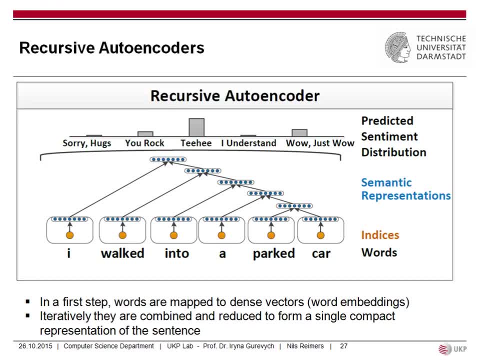 average, or either do an average over all the 100-dimensional vectors, or you do a weighted average using TF-IDF values, which is a baseline. But he presented here a bit smarter way to do it, And here it's recursive, because we map all the words and so we get a baseline. 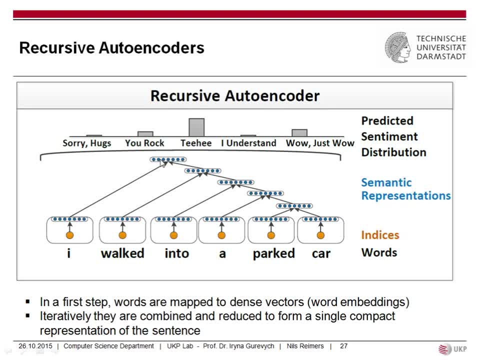 We get one single 100-dimensional output for the whole sentence. So this vector is presenting all the knowledge in the sentence And using this 100-dimensional output vector we can just add a simple softmax classifier and do some predictions. So here he had it on a. 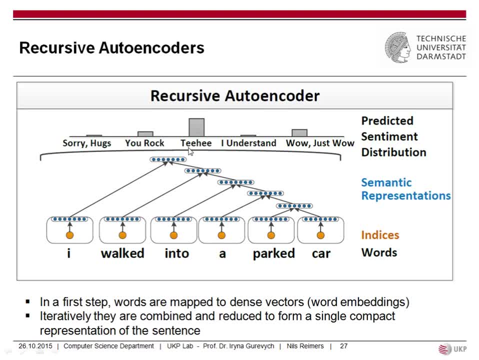 sentiment task, so where people could vote- oh sorry, Hux, you rock. Gee, I understand Well, wow, just wow. So where people could express their emotion to the statement And from this 100-dimensional output vector for the sentence, he could predict what is the. 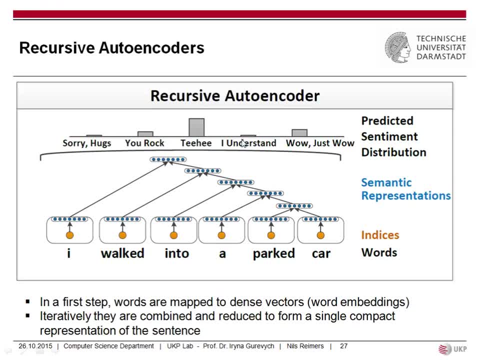 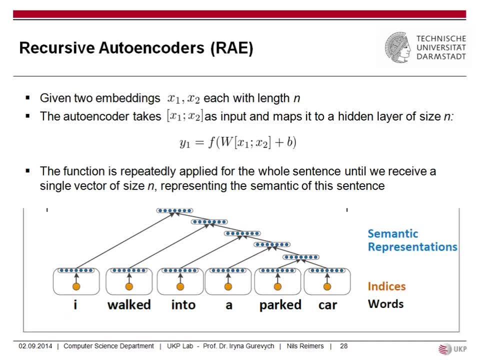 distribution. So think people wow, just wow, or yeah, it's sad, but I understand what you did. So to give you some math, given two embeddings, x1 and x2, each with the same length, 100-dimensional. 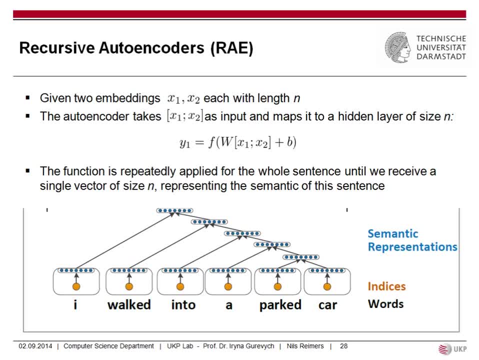 for example, the outer input coder takes these two vectors, these two embeddings, apply it to multiply it with a weight matrix w and add a bias vector b. So w and b is something which you learn during your training process And this function is repeated recursively. 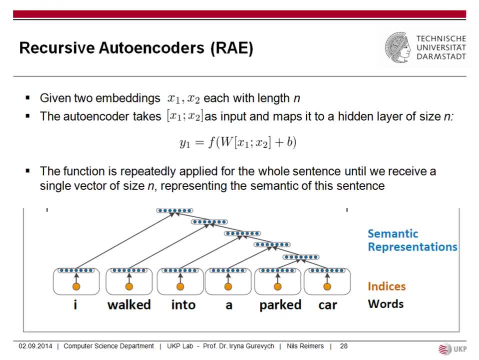 until you get a single output for your sentence. And how do you get w and how do you get b? Look at me, So you're going to use our encoder. so we have x1,, x2, v, All right, All right. 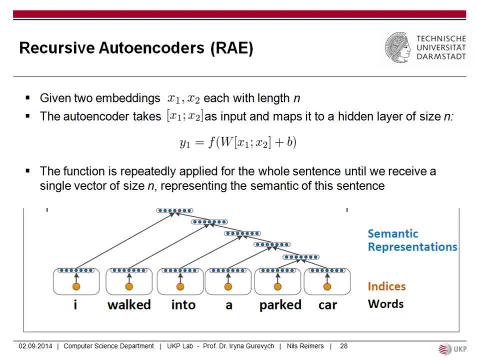 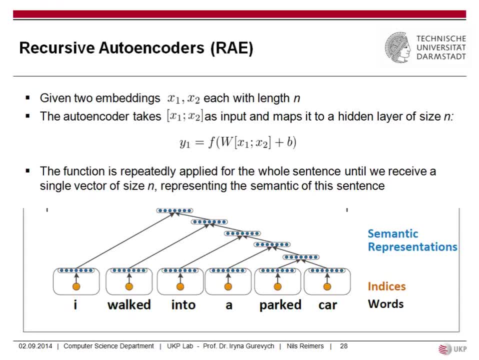 and the bias matrix vector. then you try to reconstruct your two input embeddings- and this is a step you can learn with an autoencoder, so you input just different pairs of words and learn this weight matrix w and this bias vector b, and the idea is that you try to do this compression. 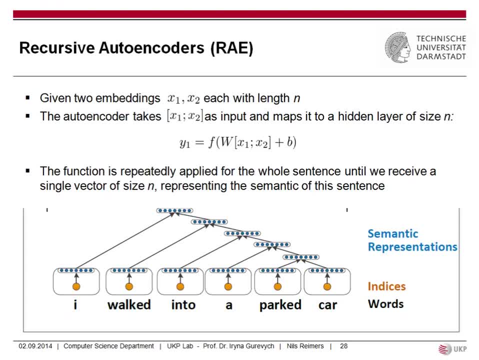 or you try to reduce the velocity of this compression, so you try to keep in this vector as much information as possible about these two words, and so you can think of what we want here. we want to have in the final vector as much information as we have in the sentence. 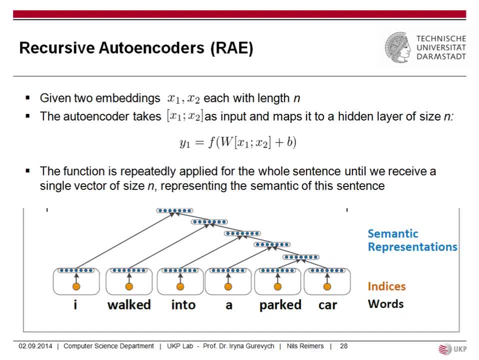 so we do not want to get an arbitrary strange information, but we want to keep the most important information of the sentence in our final embedding, and that's what you can do with an autoencoder. the autoencoder forces that you get. this 100 dimensional output contains as much information as 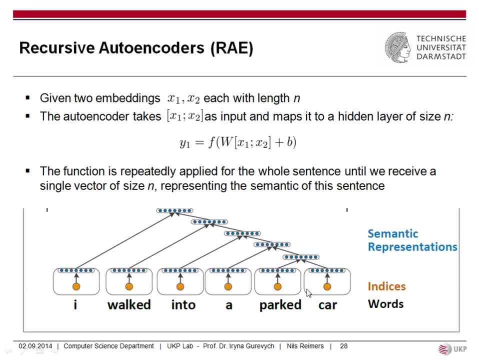 these 600 dimensional input? yeah question. so here it's right to left, right to left. you can also go left to right. so here it's just for presentation purposes. in his 2010 paper, 11 paper, he did a greedy approach where he optimized also how the tree is constructed. 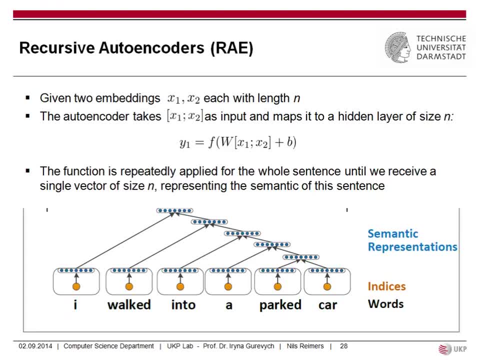 so that the reconstruction error is as small as possible. so he tried here all combinations or graph structures and see what is the output, and to make the output as good as possible for reconstructing the input, and so that's what we did here, and so that's what we did here. 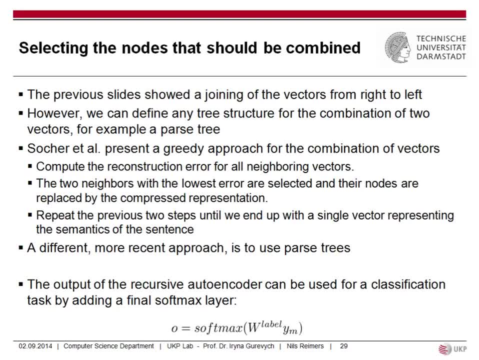 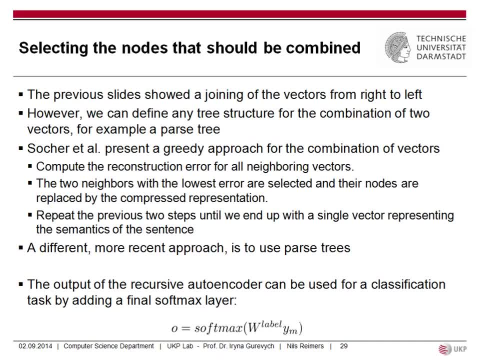 the dependency links to do combination of words. using parse tree has the advantage that you can get really sound linguistic information into your tree structure. disadvantage is that you need a parse tree and also advantage of a parse tree is that you can do annotation for the labels. so what he did on 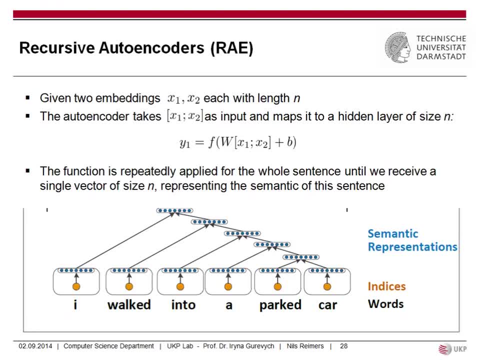 his paper he annotated positive or negative, so he took for two pairs- are these two words or is this phrase positive phrase or negative phrase? and then already trained the classifier on the phrase level and not on the sentence level. so you can see, I don't know, this was not a good move. 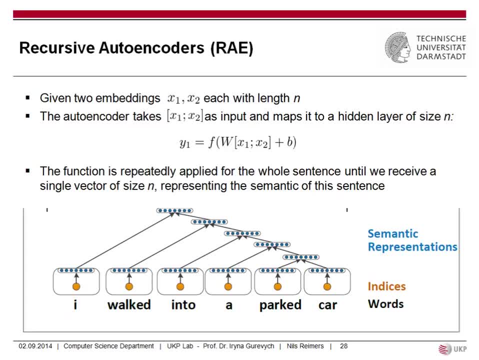 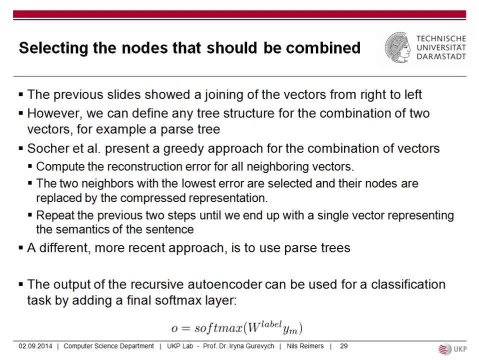 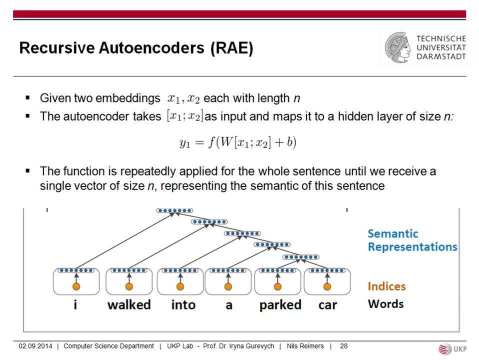 good movie would be like positive, not a good movie would be negative. and then the function this tree can learn. okay, how does negation work in a parse tree? and yet, as the last layer, we can just use the softmax function. so we have our output and then use a softmax function. 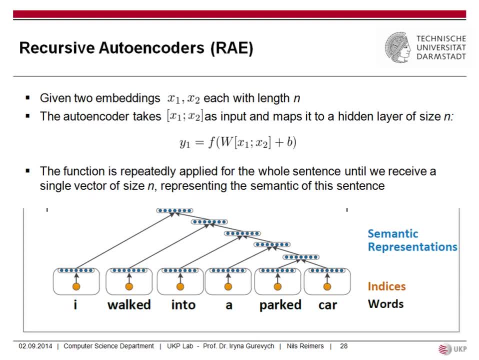 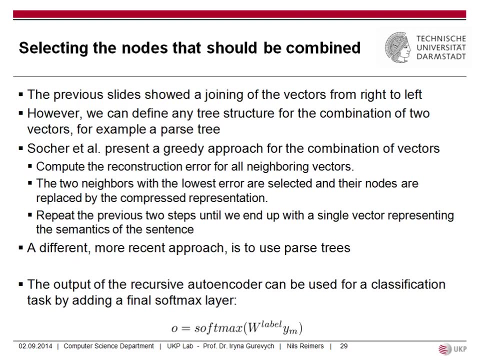 and you can do any classification task on this and it works really well on different, differently sized sentences, also on quite complex tasks. so sentiment is the most common task where you try this approach. questions on that. so I think there's no direct implementation in Keras for it. 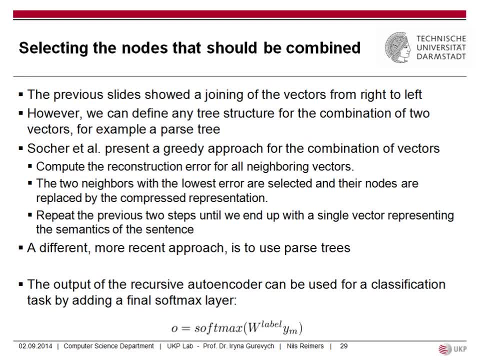 there is a java implementation from Zoffer which implements the recursive neural tensor networks, how we call it, but I haven't tried it. but if you have some sentence classification tasks, it's a model I would consider and which also gives you state of the art results, which is really nice to train and to use. 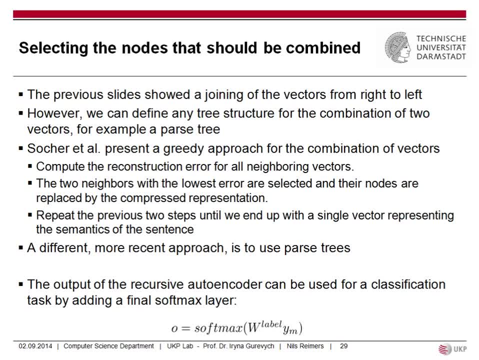 but a bit complicated from my perspective to implement it from scratch because you have this recursive thing and the maybe parse level annotation thing. so it's phrase level- sorry, phrase level- annotation thing, which is not so easy to do. basically, you would take, like, each production, you would parse the. 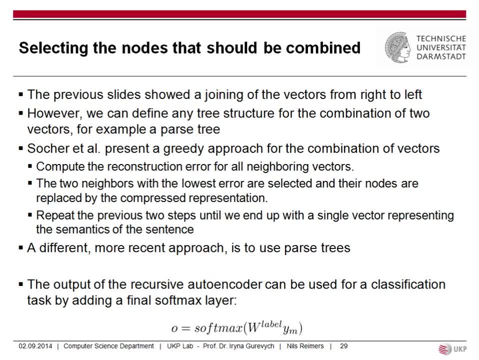 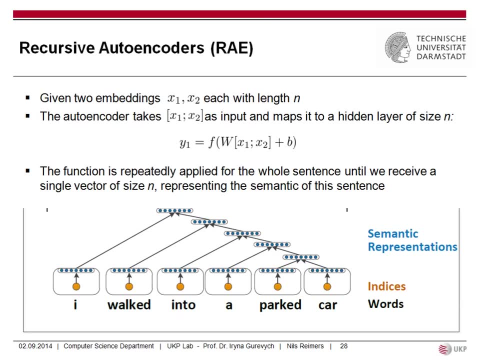 the whole focus, each production rule, you know, starting from the leads, from the contents, just joining them and doing the autoencoder for each of them. correct, you would end up with somebody. well, somebody, number, that's still huge, but yeah, basically that's it, and then you get a. 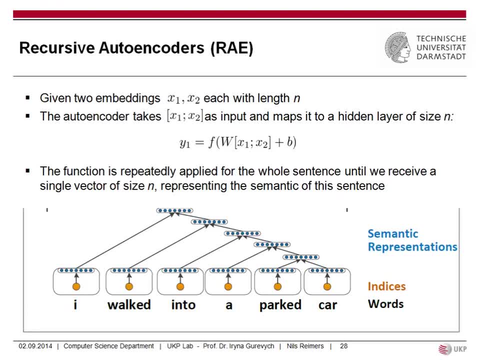 how do you apply that? yeah, and then you just add your softmax classifier with like hidden layer with the softmax classifier on it. so what's interesting to note is that we have some weight sharing, so for every combination we use the same weight, matrix W. so it 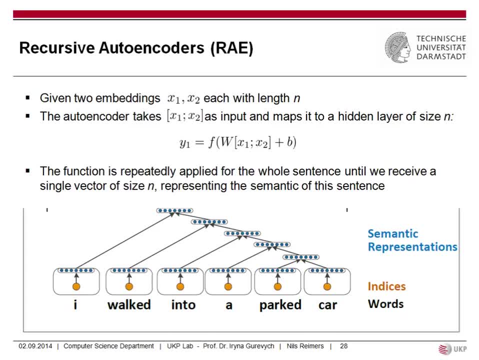 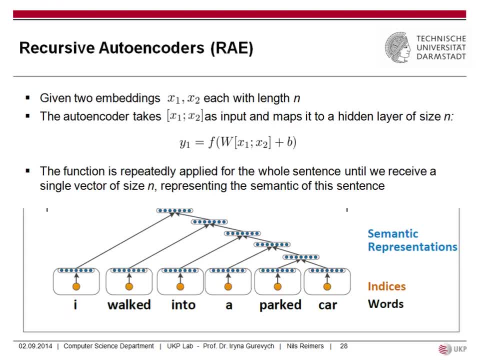 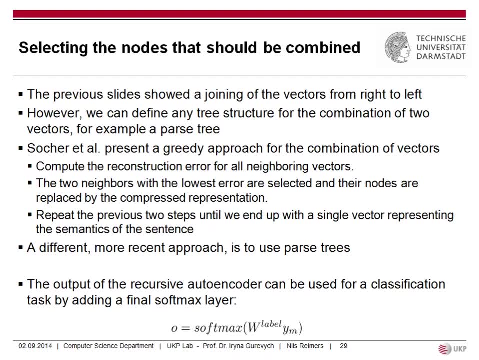 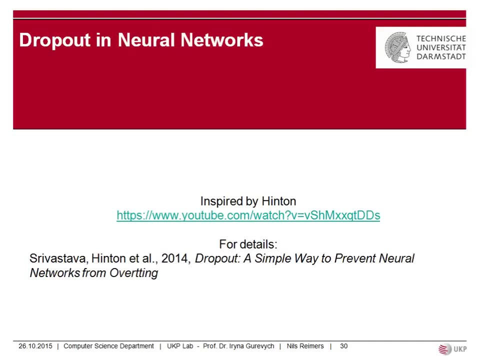 to the Jesus what there are. recursive autoencoders- really nice model, Really. also look into the papers of SOCHA. They are, I think, quite easy to understand, quite easy to read, and you can use it for like a lot of different tasks. 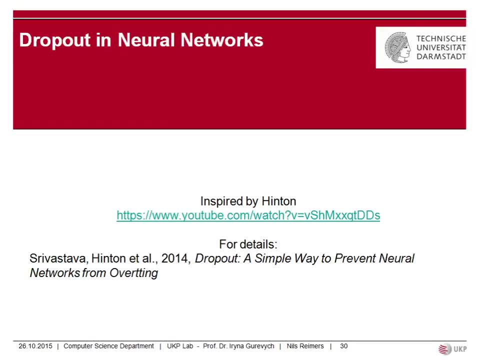 as you've seen with the co-referenced resolution, where we use the same structure as for named entity recognition and part of speech. You can use this for all sentence classification tasks. Now I'm going to talk about dropout in neural networks, and I stole the idea from Hinton in his lecture he gave. 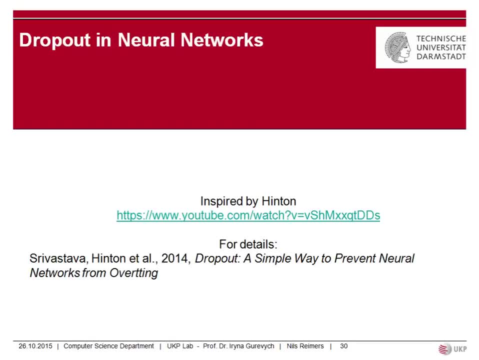 You can find it on YouTube And if you want to have more scientifically results on it, look at this 2014 paper Dropout: A Simple Way to Prevent Neural Networks from Overfitting. So ensemble learning. So who knows what is ensemble learning? 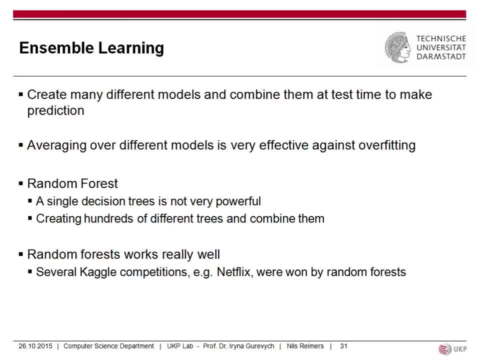 You want to explain it, India? Yeah. so basically, ensemble learning is when you have like, instead of training one classifier, you get several classifiers and you modify. so it depends on the method, but basically you train several classifiers in your data. 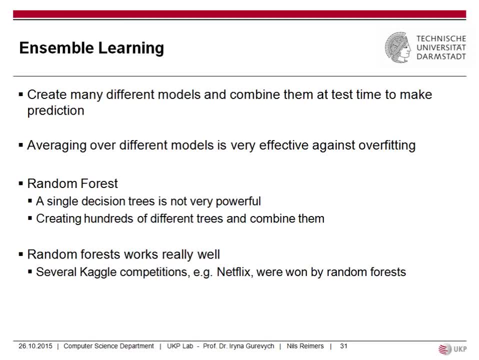 by modifying the classifiers for your data a little bit and then you combine the results from those classifiers using some weights and you have another. as far as I understand, you have another meta classifier that uses weights from those classifiers to produce final classifier. 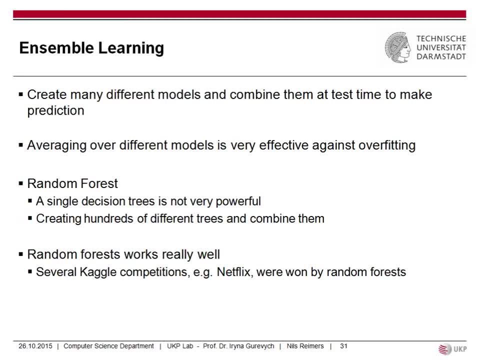 Yeah, so you can use a meta classifier or you can just compute the geometric average, And the idea is you create as many different models as possible and you combine them at test time and you average over the different models and this gives you a very effective method. 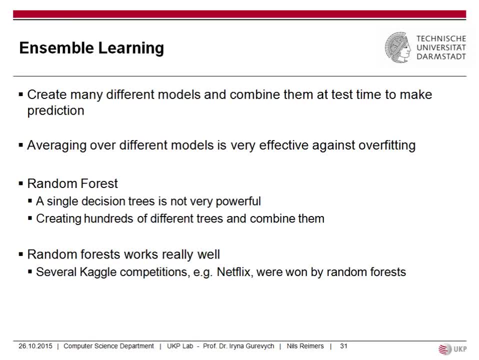 against overfitting, because your one system, your one life-based classifier maybe overfits, but your support vector machine does not overfit on some things and there's one model called random forest, so it uses decision trees. Decision tree is like a really bad model. 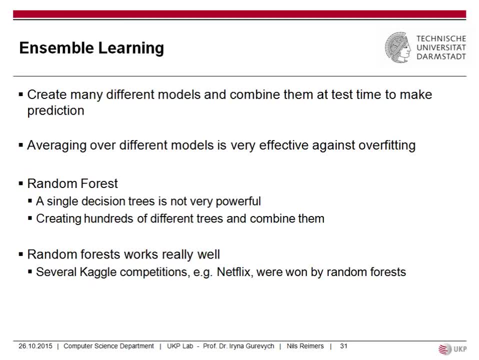 It's not really working so good, but in a random forest you initialize, for example, 100 or 1,000 different decision trees and you average over the output of your 1,000 decision trees and random forest works really really well. 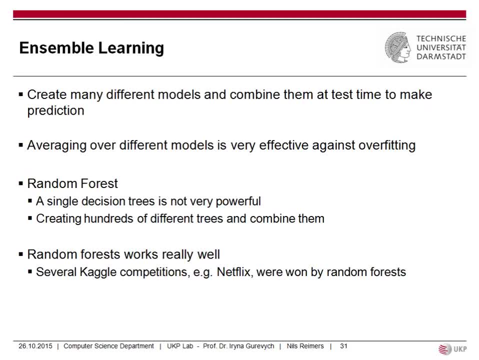 so there are a lot of competitions. so, for example, the Netflix competition which tries to predict which movie would you like to watch next, which is like a good movie recommendation, really big data set and was won by random forest. and when you go into the data science community, 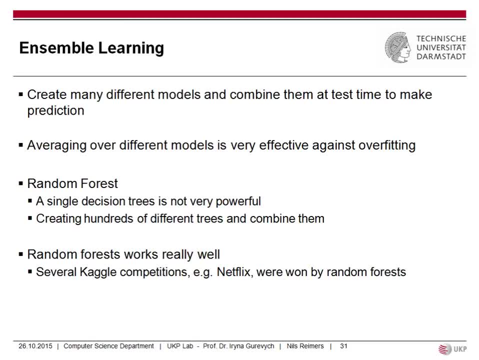 you see that a lot of people win competitions with random forest and the trick is: okay, you have like really bad, simple classifier decision trees which is easy to train, but when you combine a big bunch of them you get a really good predictive model. 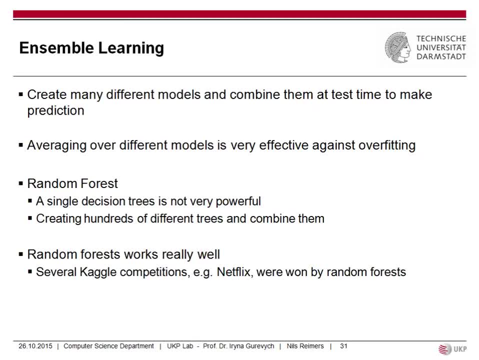 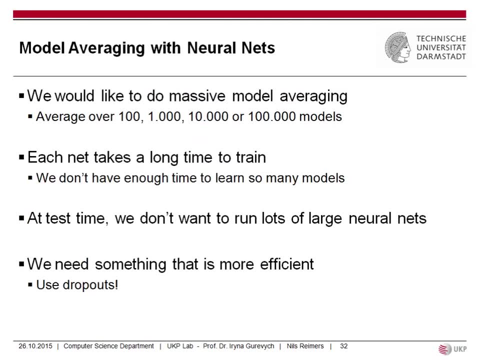 so it's like swarm intelligence which we use here. so we use a lot of classifier with our stupid, but as a swarm they are quite intelligent and give you really good results. So what would be great to have this also neural networks. 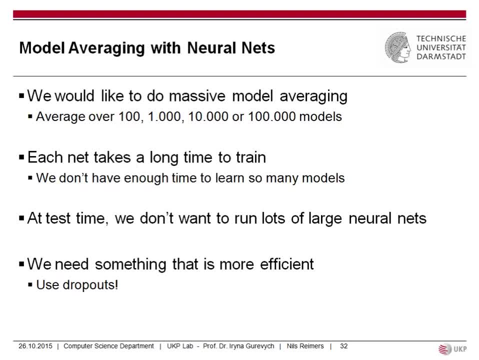 so we would like to do massive model averaging so we would average over. I don't know, maybe we'll start with 100 different neural networks, or even like could also imagine that we average over 10,000 different neural networks, where we train on it and we hope okay. 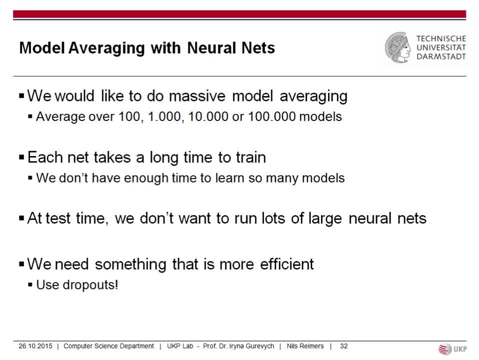 when we take 100,000 different neural networks models into account and average over them that we get like really awesome results. Problem is that each network takes a long time to train. So I mean when you tried the experiments? 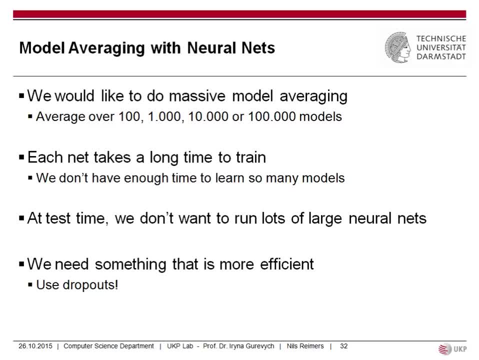 even on small data sets, on simple examples as hand-fledged and digital recognition. you see, it takes really long time and we don't have enough time to learn so many models. so no one wants to train 100,000 models And at test time of course we do not want to compute 100,. 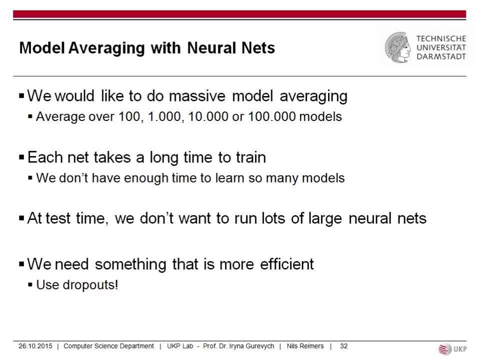 the output of 100,000. So we want to do the average, so we need something that is more efficient and we use dropouts for that, which is, like, from a mathematical point, really crazy but a really beautiful idea. 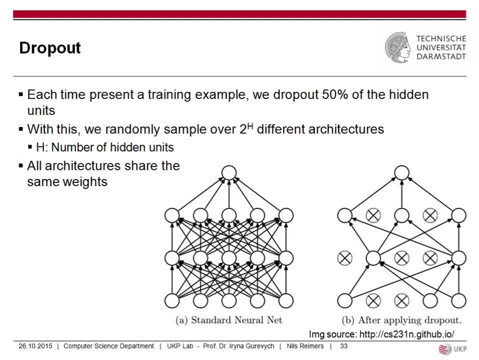 So what is a dropout? Each time you present a training example, we drop out, for example, 50% of the HIN units. You can also change it to other numbers: 10%, 90%, but 50%. so you have like flip a coin. 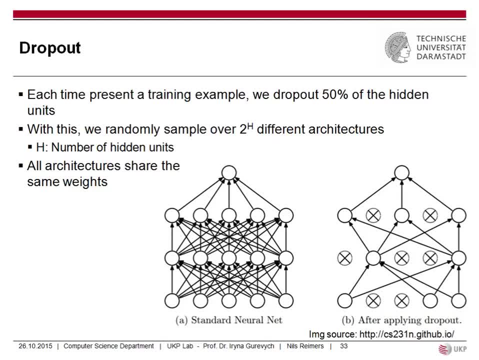 should the HIN layer, the HIN neuron, stay in the network, And in a normal fully-connected feedforward network, it would look like something like this: So you have here your three HIN layers and it's fully-connected, and then you have your output here. 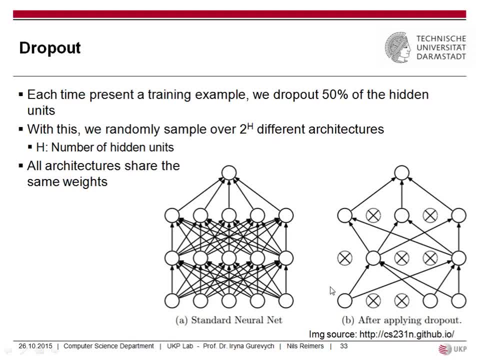 And after applying dropout, you go in every layer and arbitrarily it shows with a 50% chance. okay, you should live or you should die. So here we say, these two models we set OK, set it to zero, taking it out of the model. So when the value of a neuron is zero, apply zero. 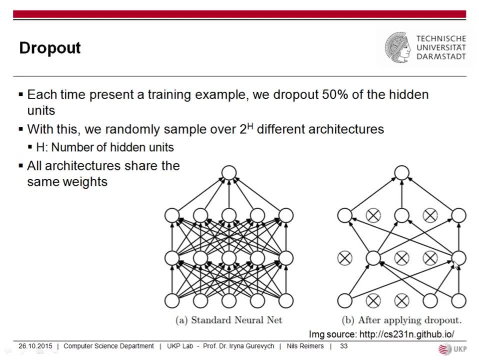 times the weight, so it does not have any effect. And you do it for every layer And our final model would look like this. So here we deleted two nodes, so we have some connections here, and then we have some connections here and some connections here, And when you do the math you get the crazy number. 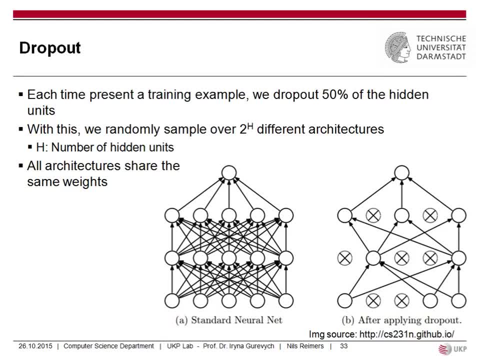 that you randomly sample over 200,, 2 to the power of h different architectures and h is the number of hidden units. So when you have like 100 hidden units in your model, and so they're 2 to the h, so 2 to the power of 100 different architectures And, what's important, all architectures share the. 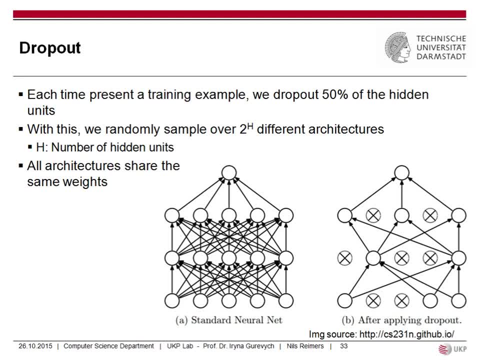 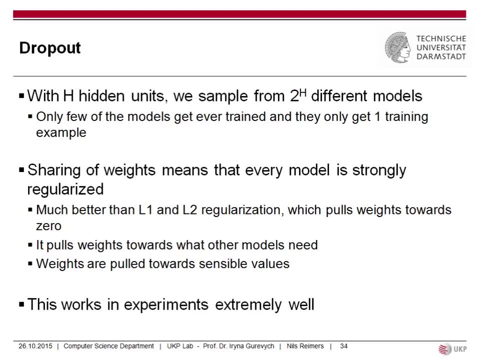 same weight. So this is like the idea of dropout. So what's really crazy is when you have like h hidden units, you sample from 2 to the h different models. Every model gets few or only few of the models get ever trained. So 2 to the 100 is a. 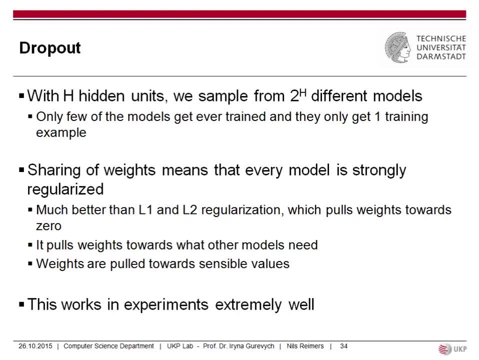 really large number. It's extremely large And every model we train is only one. get one training example. But sharing the weights means also that every model is strongly rectalized, So it's much easier to do the same thing. So we have an L1 and L2 regularization which pulls weights towards 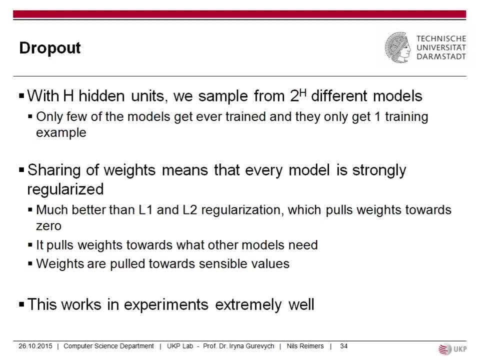 zero. So dropout pulls the weights towards what other model needs and the weights are pulled towards more sensible values. So L1 and L2 regularization to give you some background on that, so you ensure that the weights get not too large, Because when the weights gets too large, 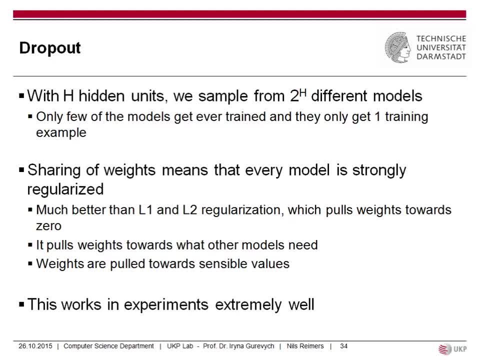 your model overfits. So, for example, for handwritten digit recognition, it detects that the pixel at the lower left corner it's like, really important to predict an 8.. Because in your training time there was a single or this pixel was only active once and it was an 8.. And so 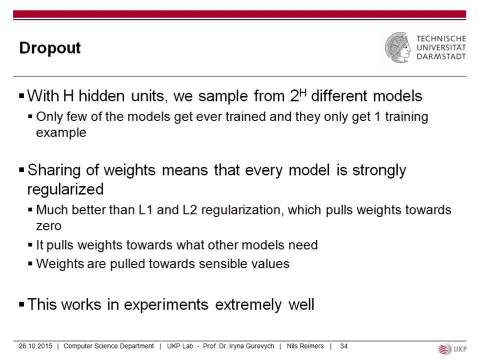 your model thinks: okay, when this pixel is on it's always an 8,, which is, of course, garbage and where you fail in test time because of overfitting. So you ensure it usually was L1 and L2 regularization With that that it's not overfitting. 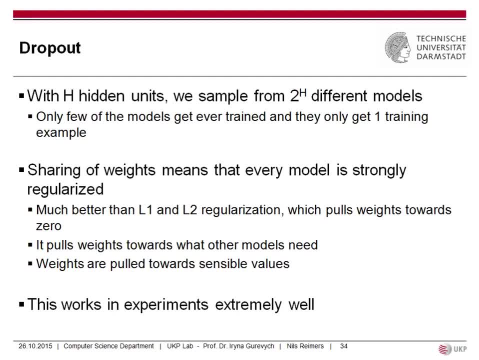 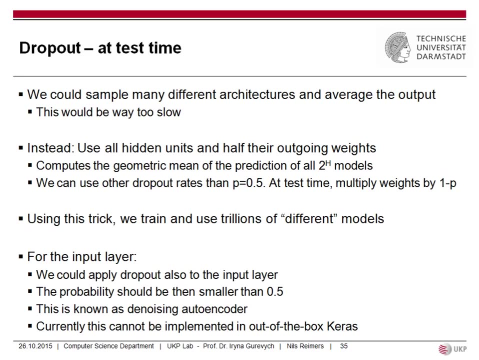 And using dropout is like, more, more suitable to, to to ensure that overfitting is not working or not not happening. So at test time we could sample many different architectures and average output. So we could- I don't know- use dropout several times, and then we get different. 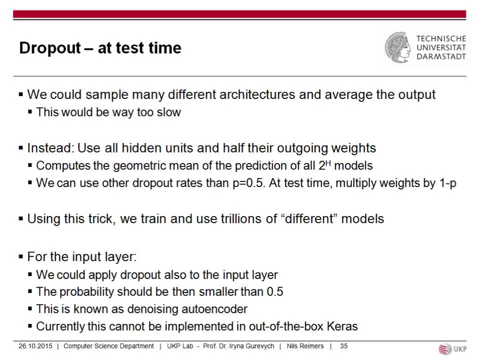 combinations of our hidden units and then get the output And average them, But instead for test time we use all hidden units and half the outgoing weights. And what's really really crazy is that it computes a geometric mean of the prediction of. 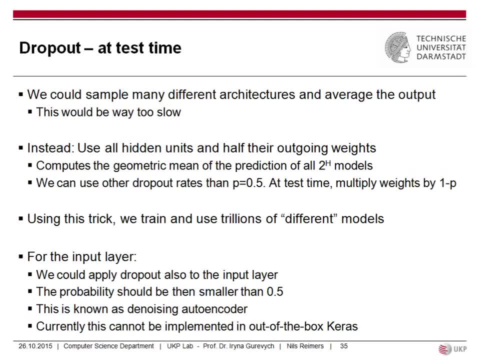 all two to the H models. So when you have 110 units, you get predictions from two to the H models. so two to the power of 100 models, which is like trillion. So you get the prediction of trillion different models. you have to do a geometric mean. 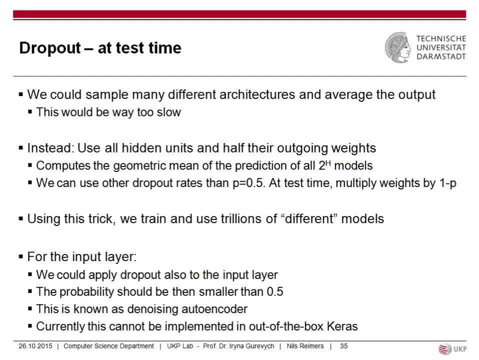 And we can easily use a dropout rate of p0.5. if you use a different dropout rate, you multiply the weights by one minus p And we use. you can use this really simple trick and you get like the output of really different, a lot of different models For the input layer. you could also apply the 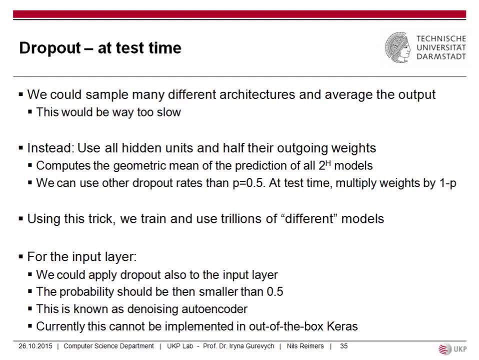 dropout for the input layer, but the probability should be smaller than zero- 0.5.. This is known as denoising autoencoder, which is a bit older model, but people nowadays only apply it for the HIN layers and there's also no implementation in Keras, where you 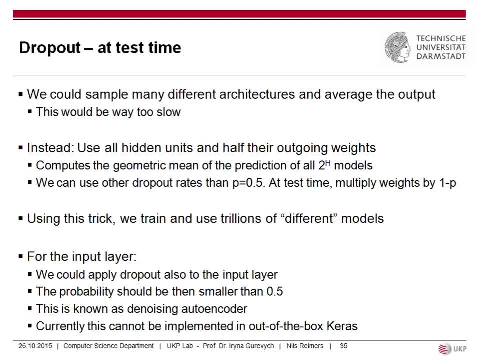 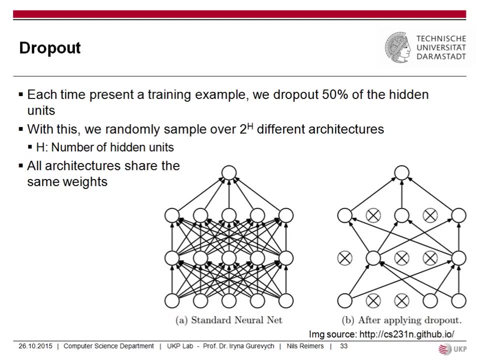 could drop out some of the input units. Questions on that. Can you go back to this slide, This one, Where we had, yes, two to H, So we have sample over two to H the architectures, but it's less than two to H, okay, Sorry, say again. 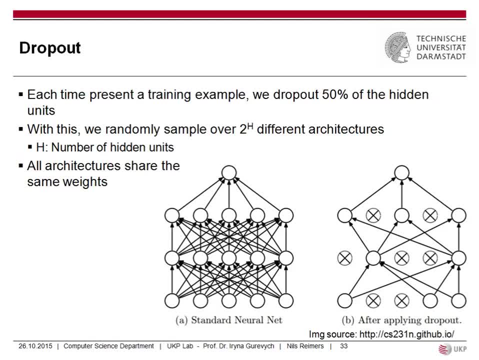 Our sample size is less than this explanation. Okay, So when you drop out 50% of your HIN layers, you could think of: you get. You get two to the H different networks, because this is one network architecture, and then 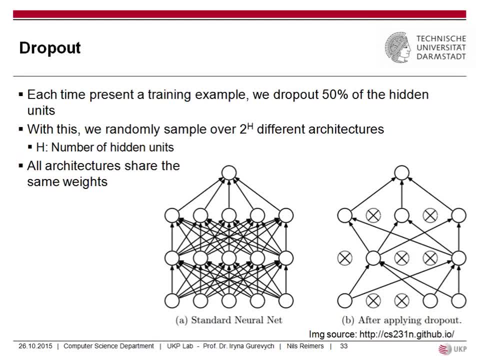 you. I don't know, in the next run you drop out other layers and it creates a different architectural layer And there are two to the H different architectural layers when you use like a dropout of 50%. So there are like two to the H different possibilities. 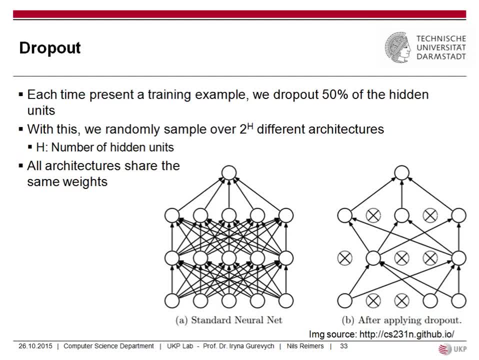 how your network, how the connections could look like when you use dropout 50%. Oh, okay, Yes, okay. And when you use this, it's the same as you do compute the geometric mean of two to the H different models. So it's the same as if you would compute or train two to the H different. 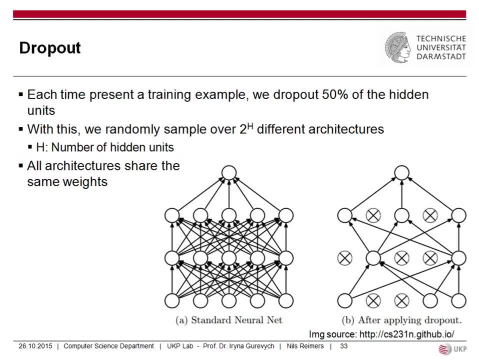 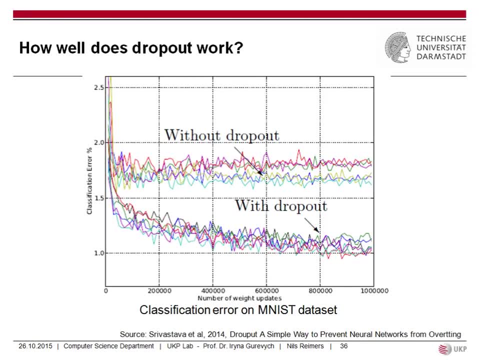 neural networks from scratch, like this, and then do a geometric mean for the output. So how well does a dropwork out work? So this is the classification error on the MNIST data set And with dropout we get an error which is, I don't know, 1.6 without dropout. And 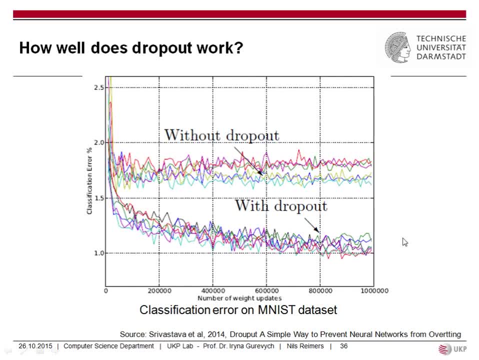 with dropout, it decreases to like 1.1.. So, which is quite, quite big. Other architectures, other papers report on that. they get, for example, for the F, for the sentiment- prediction is a sentence positive or negative in sentiment- that the accuracy increases by two. 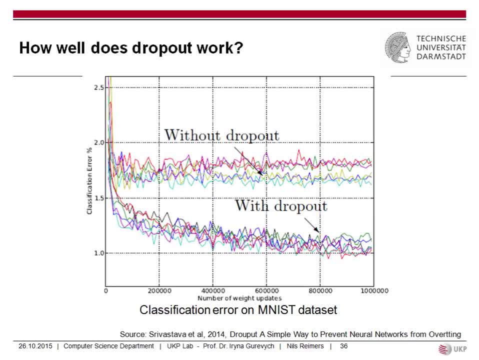 Up to 4% in accuracy. So it increases from, for example, 70% accuracy to 74% accuracy just using adding a dropout layer. The first one, the no-dropout, is regularized, or is it just? I think it's regularized, but for details, I think the first one is regularized. 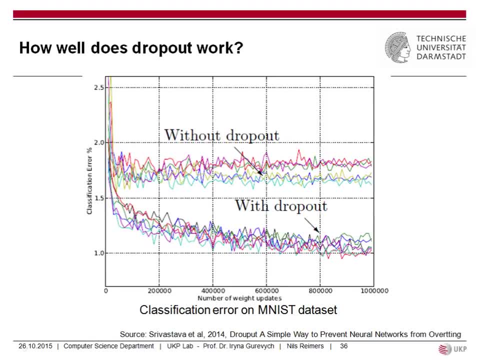 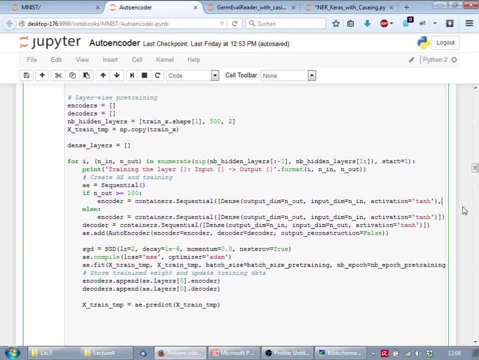 Okay, Okay, Okay, Okay, Okay, Okay. So it's easy to implement. There's one, one command in Keras where you can just add a dropout. So it looks something like this: So you have your dense model and then you can just say you had a dropout. 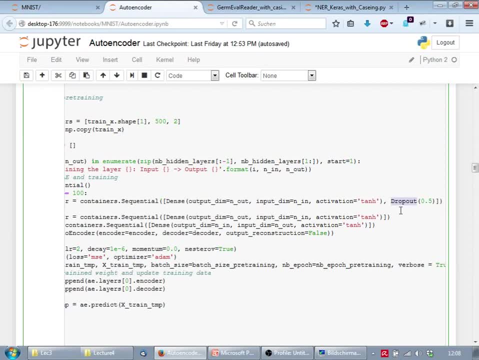 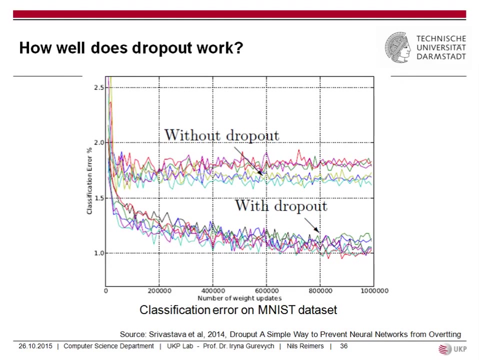 So you have a dense model and then you add a dropout of 0.5. 0.5. 0.5. 0.5. 0.5. 0.5. 0.5. And that's how you get your dropout layer into your network, which prevents overfitting and increases your QLC. 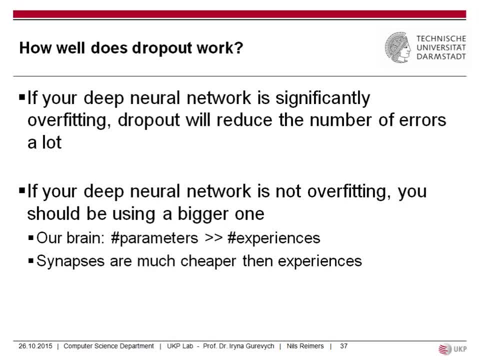 So the recommendation by Hinton in his lecture was if your deep network is significantly overfitting, dropout will reduce the number of errors a lot. So if you fail due to overfitting, try a dropout layer. And he also recommends if your deep neural network is not overfitting you should be using a bigger one. 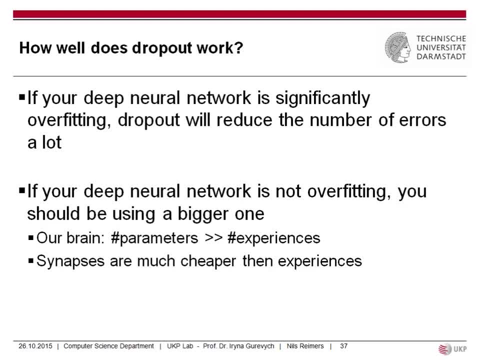 So add more HIN layers and increase it, and increase even more HIN layers, and increase even more HIN layers until it overfits, And then you can add a dropout for it. And the theory is that, for example, in our brains, 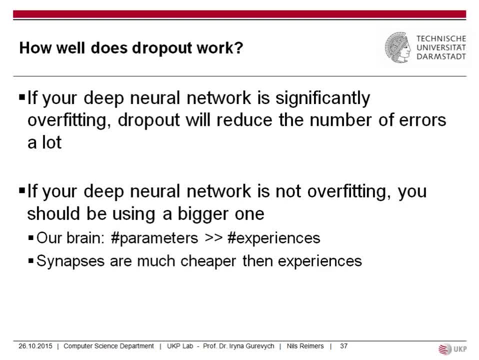 we have a lot of more parameters than experiences. So we have a lot of synapses in our brain, So many million trillion synapses in our brain, But we have only quite a number of experiences. So our lifetime on Earth is quite limited. 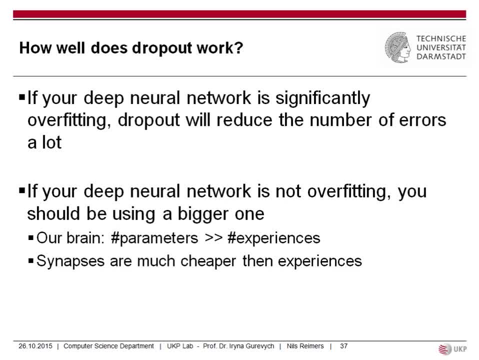 And we have a lot more synapses in our brain than we have lifetime. So it seems when you look at the brain that it makes more sense to have more synapses, More parameters and to try to increase the experiences. So you can also try that you go not from like the bottleneck where you go in the outer enclosure from a big layer to a smaller layer. 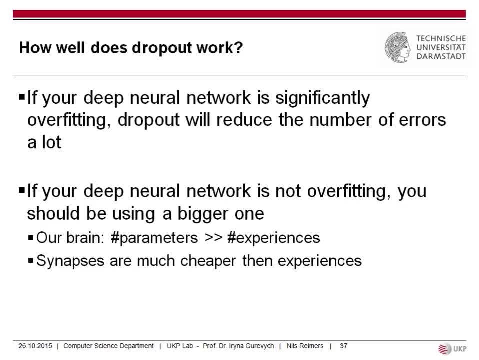 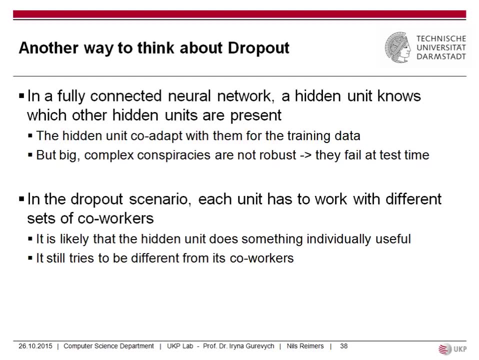 but where you go from the input layer to even a bigger layer. So let's say you start with 500 dimensional input and then you go to 1000 dimension, but you add some dropout to it- Another way to think about dropout. So in a fully connected neural network. 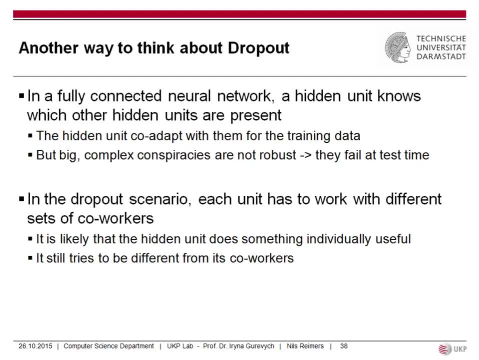 every hidden unit knows which other hidden units are present, So the hidden unit can co-adapt with them for the training data. But this creates big complex connections between and they are not robust. So it's like really really complex. They learn like really really complex rules to work well on the training data. 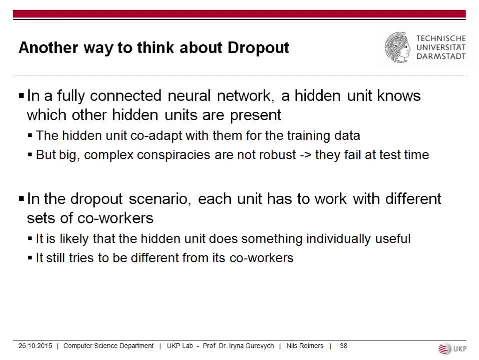 And of course, at test time they fail because the environment changed In the dropout scenario. the environment has to work with different set of co-workers, So the hidden layer does not know next time which are like my co-workers and they cannot co-adapt to the co-workers. 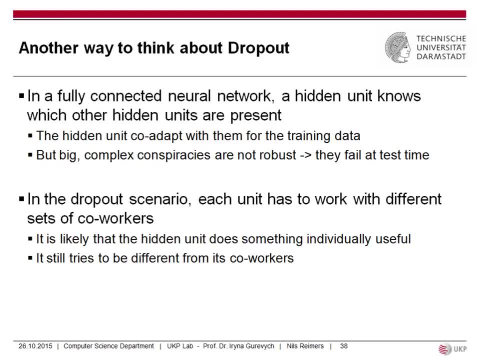 So it will force the hidden layer, that every unit, every neuron in your hidden layer, learns something individually useful and but still tries to be different from its co-workers, to still adapt some value to the new set of hidden units which are present. Okay, that's it for today. 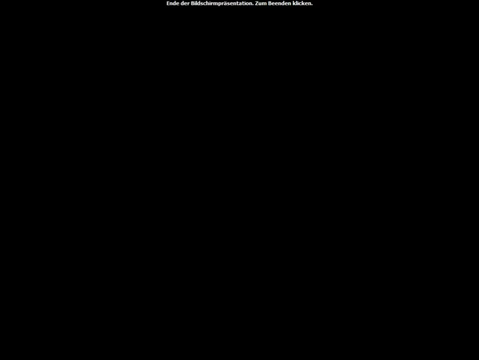 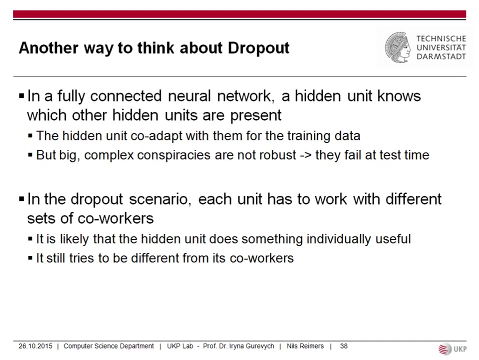 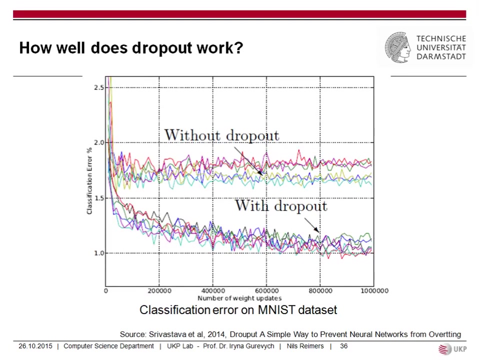 Any remaining questions? Yes, What does dropout need with the training data? So, will I need more training data or less training data, or more? It gives you, with the same amount of training data, better results. Or, when you put it, a different way,